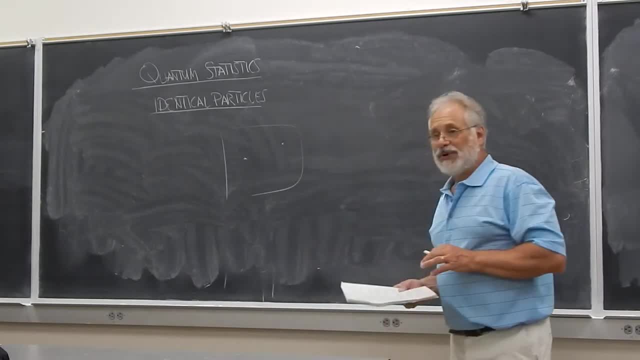 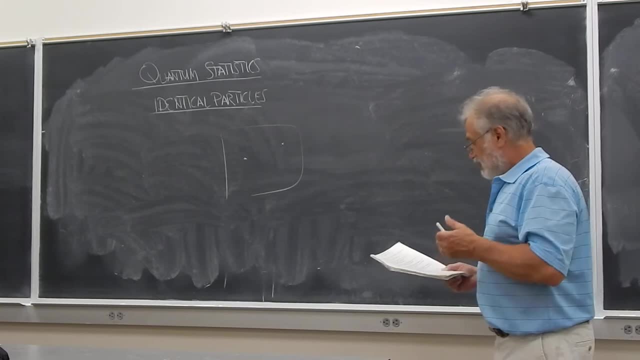 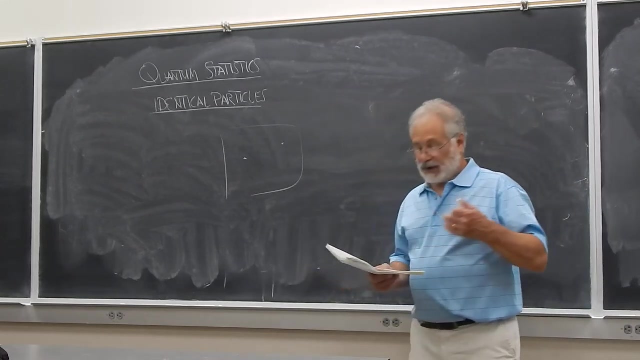 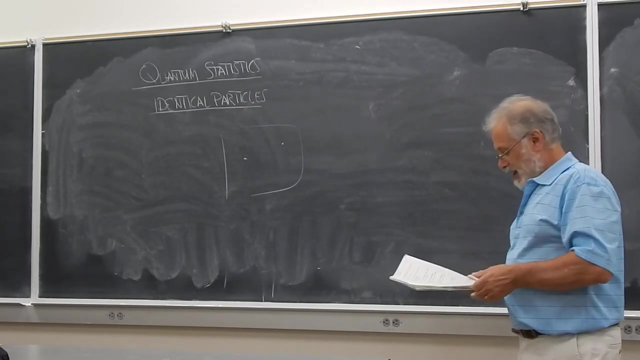 happen. For one thing, the uncertainty principle forbids us from constantly observing this, because as soon as we observe the electron, we affect its motion, In other words, we shine a light on them. they're going to be affected, But more formally than that, because of the finite extent of the wave functions associated with each electron. there may be an overlap between the wave functions. This is going to make it impossible to distinguish one electron from another. In the case of the helium atom, for example, helium has two electrons. the wave functions of both electrons can overlap very highly in all states. 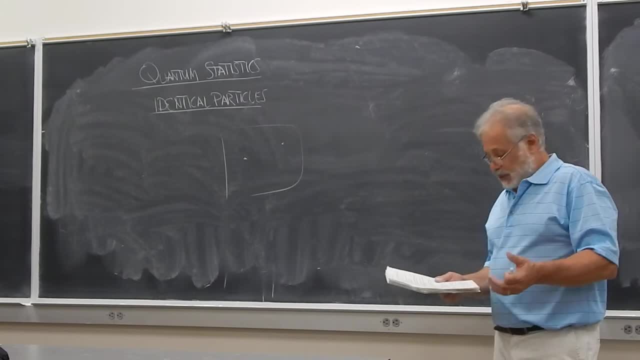 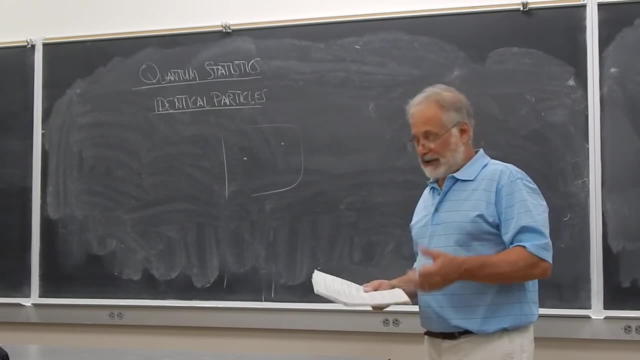 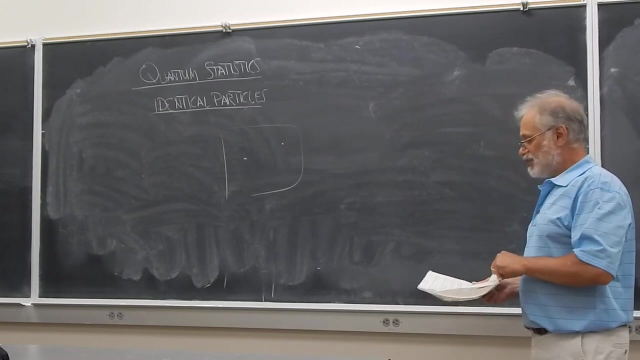 And I can't distinguish one from the other. In the hydrogen atom there's a fairly large overlap between the wave function of the proton and the electron. but that's not a problem because I can tell a proton from an electron. They're not identical to one another. 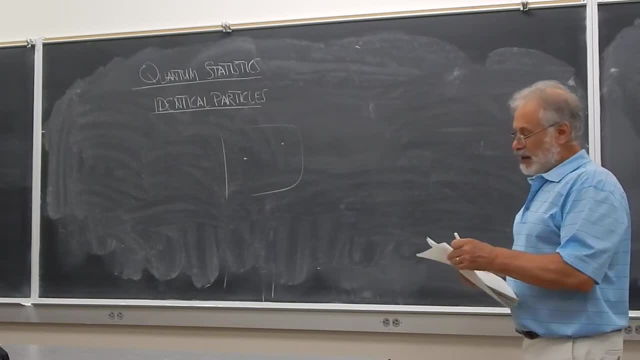 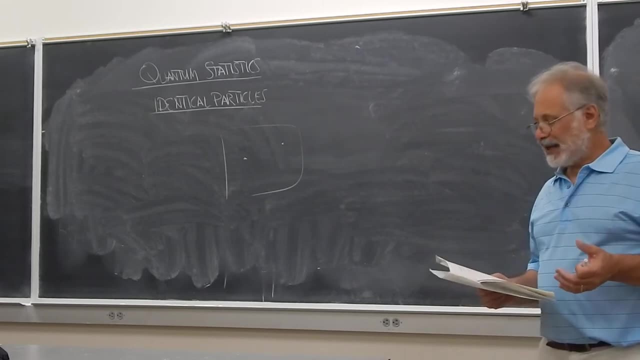 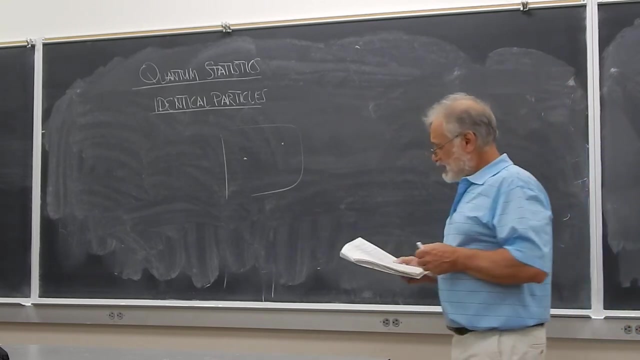 Thank you. So the idea is that any measurable results that we get from quantum mechanics can't depend on being able to distinguish one electron from another or the fact that we would have to assign labels to individual particles. So this is what I'd like to do. 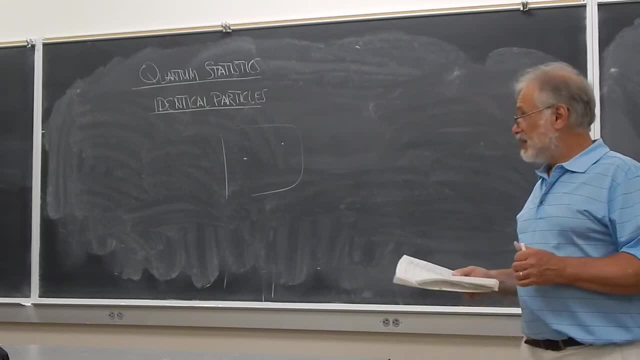 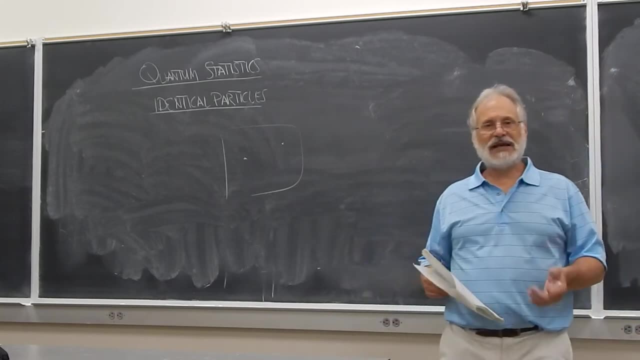 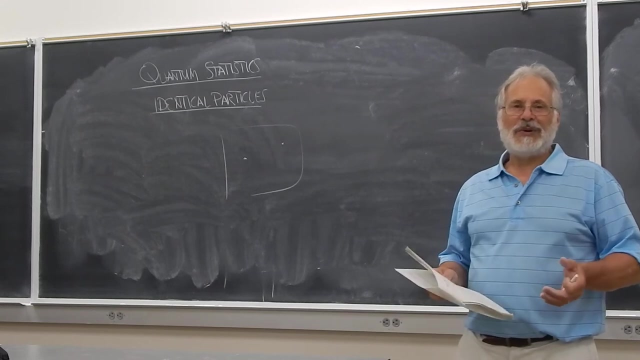 Let's write down the Schrodinger equation: These two electrons in the box. Now, yes, we're going to say the electrons are indistinguishable, but we have to find a way to label them. So, even though the labels are sort of bogus, 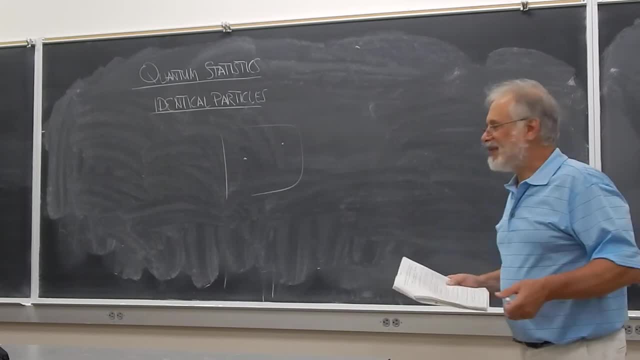 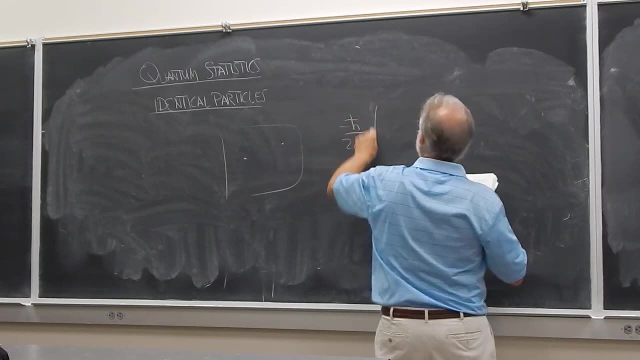 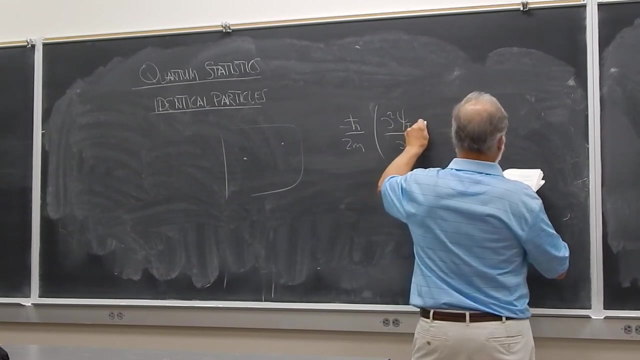 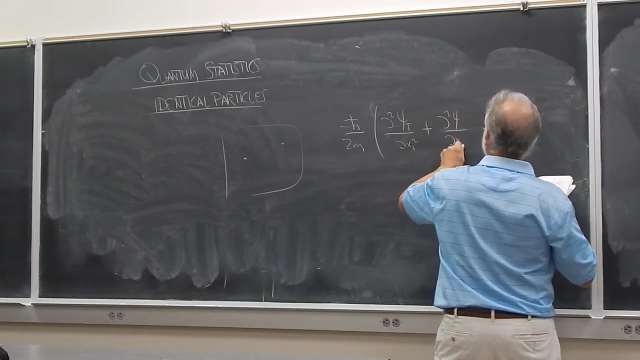 we have to use them, otherwise there's no way to mathematically describe this sensibly on the blackboard, So I'm going to write down the Schrodinger equation for this system. So this is theweek that we have buf fdp. 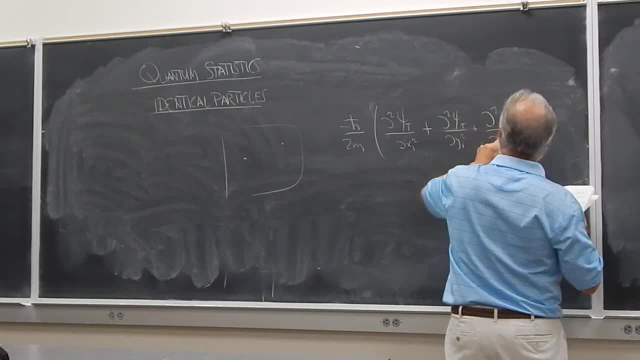 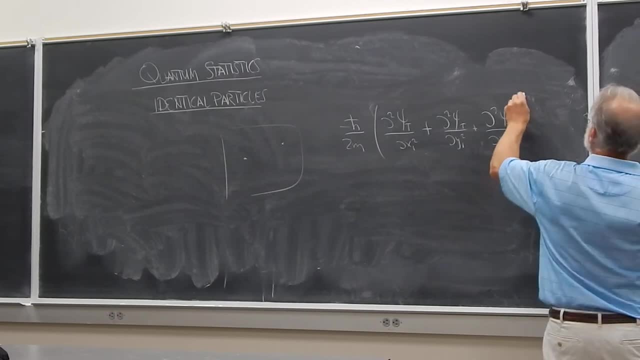 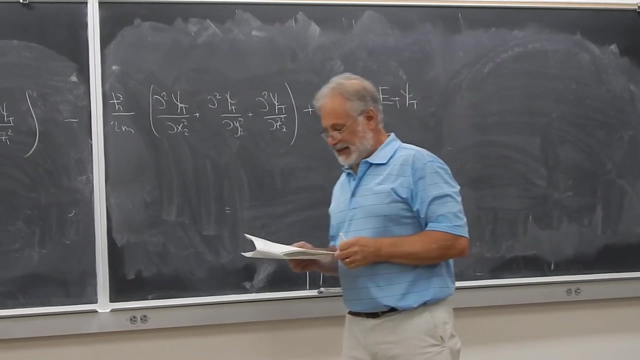 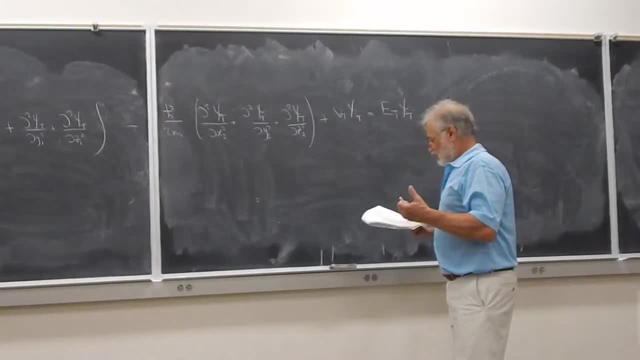 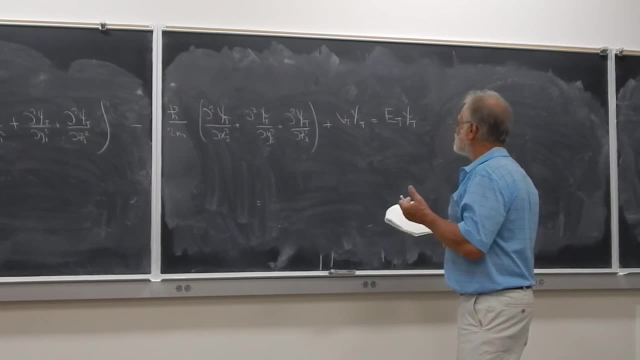 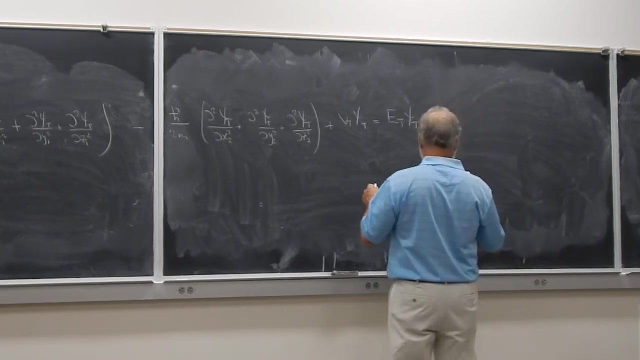 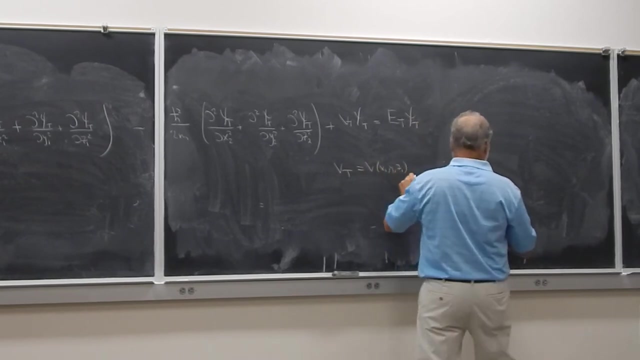 That would include spin and position the whole nine yards. Let's make some other approximations. Since the particles don't interact with each other and they move independently, their potential energies can be separated. In other words, I can write vt as v of x1,, y1, z1, plus v of x2,, y2, and z2.. 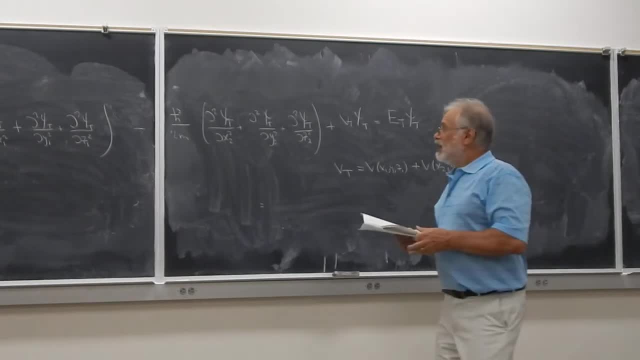 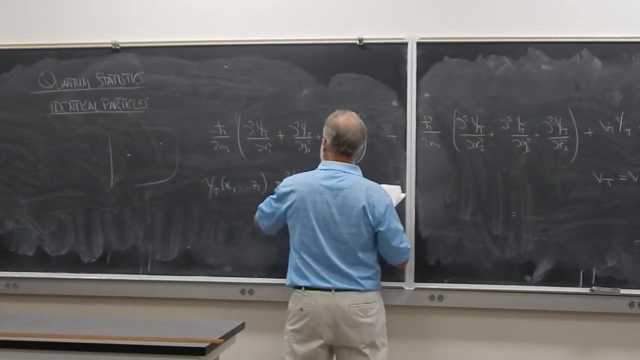 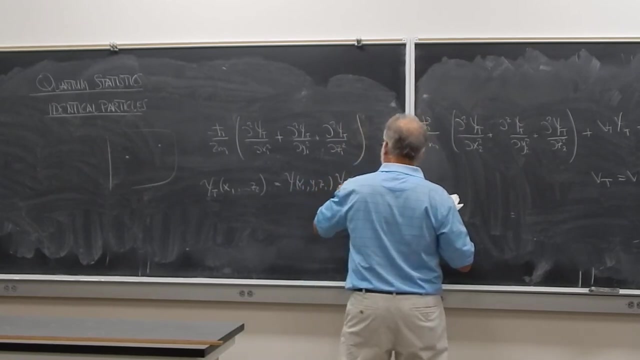 So I don't have to worry about that. Now for particles in a box. we know that the solutions of the Schrodinger equation look something like this: Psi, total of x1 all the way through z2.. I can write as Psi of x1, y1, z1, times Psi of x2, y2, and z2.. 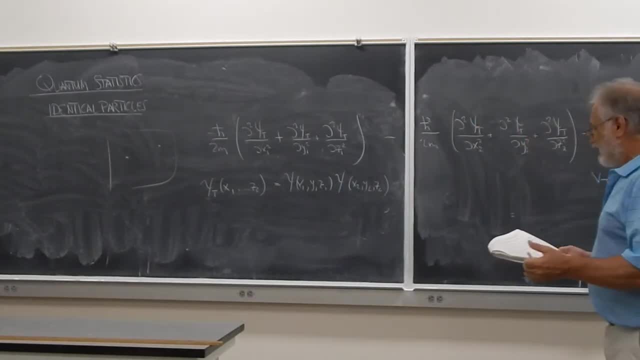 So the solution would be the product. The total eigenfunction is the product of the eigenfunctions for each of the individual particles or electrons. Now, each eigenfunction also requires a specification of the spin of the particle, And so what we're going to do is we're going to let our subscripts- alpha, beta, gamma, et cetera- represent the total state of the system. 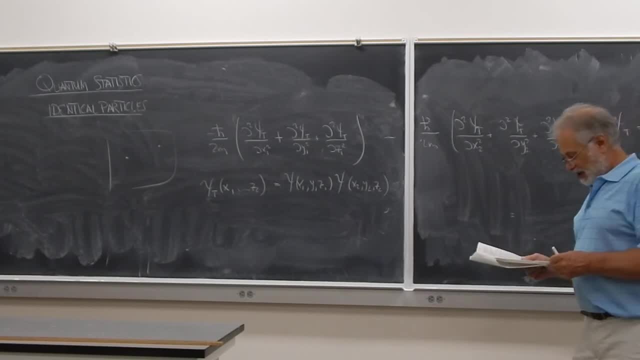 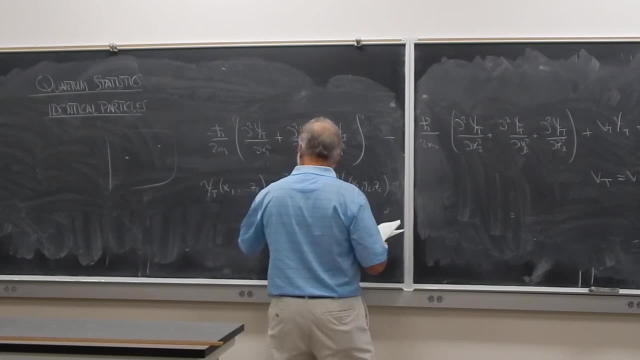 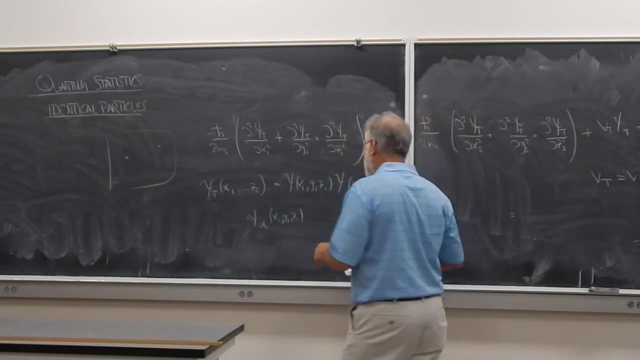 That is to say the space and the spin of the particle, So an eigenfunction for particle. one might be Psi sub alpha of x1,, y1, z1.. For the other one it might be Psi sub beta of x1, y1, z1. 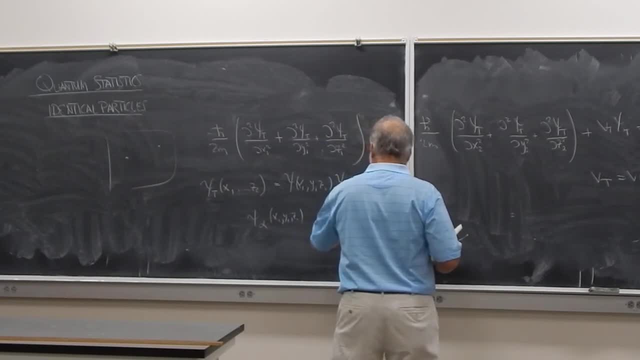 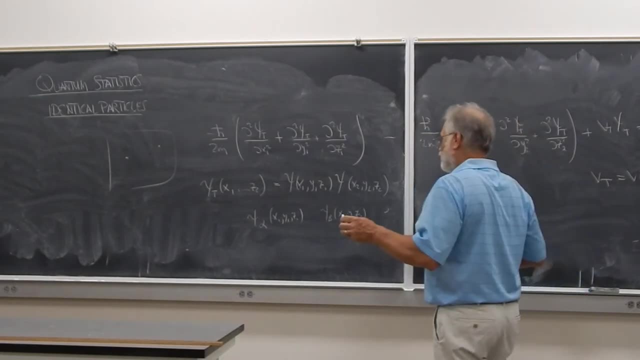 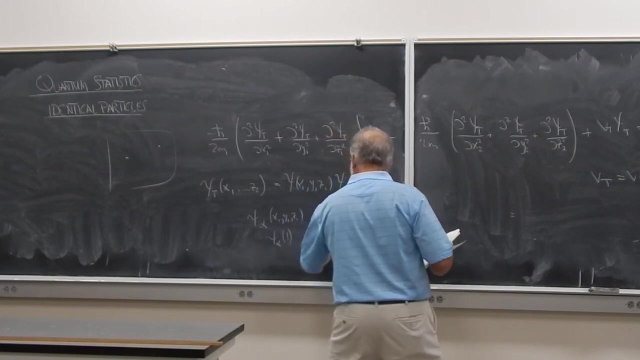 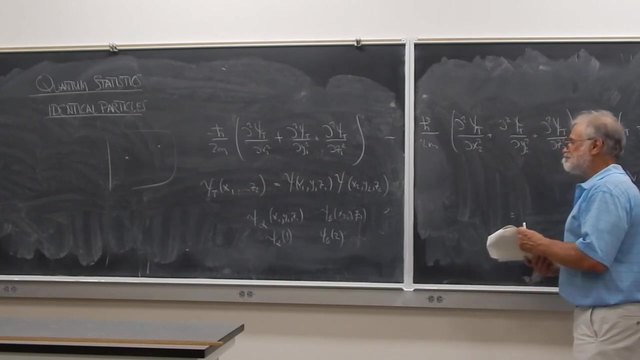 Psi is the total of x2,, y2, and z2.. And just to make the writing simpler, we'll call this guy Psi sub alpha of 1.. We'll call this guy Psi sub beta of 2.. So we're not writing all kinds of letters all over the place and making things confusing. So, in this case, to make all of this easier, we're going to write Psi. So, in this case, to make all of this easier, we're going to write Psi, sub alpha of one, And then we'll call this guy Psi, sub alpha of two. 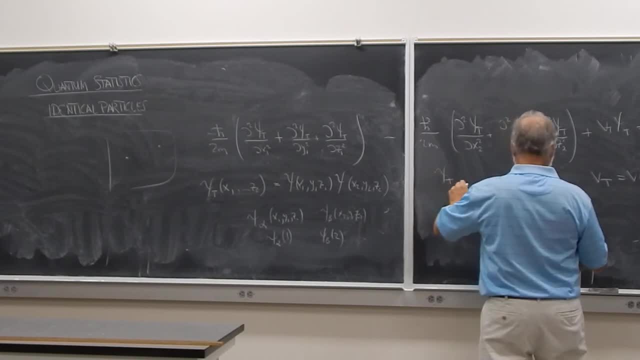 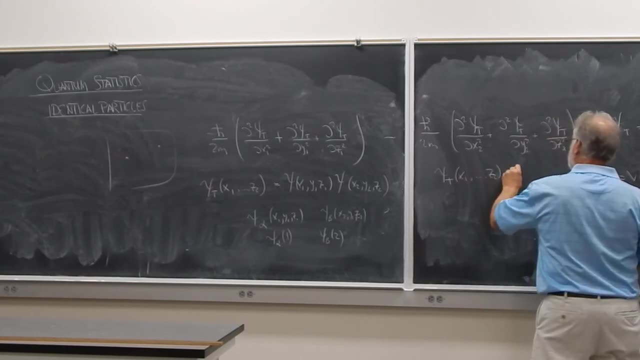 And then we'll call this guy Psi sub alpha of two. To make it short, I can write psi sub t of x1 through z2.. It's just going to be written as the product of psi sub alpha of 1 and psi sub beta of 2.. 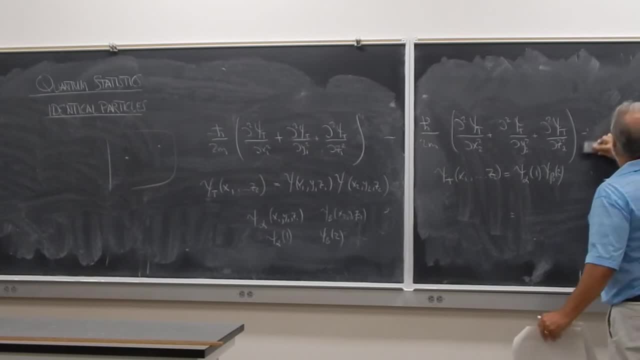 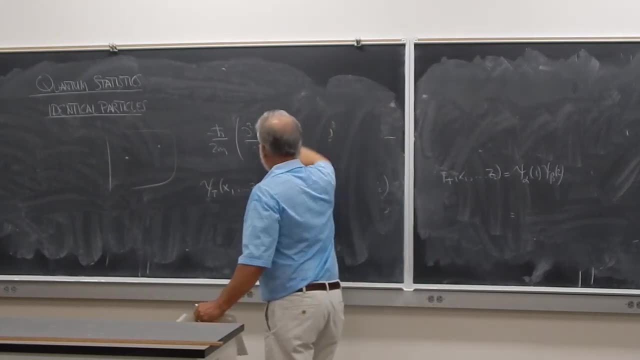 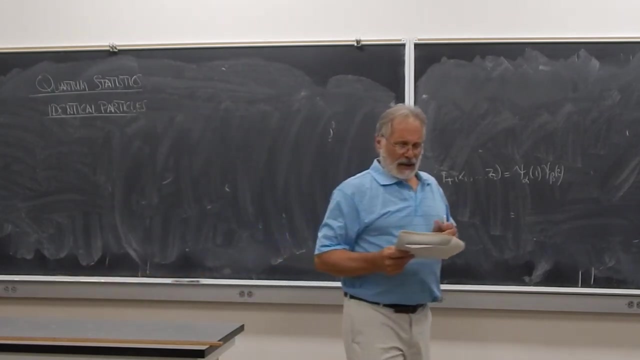 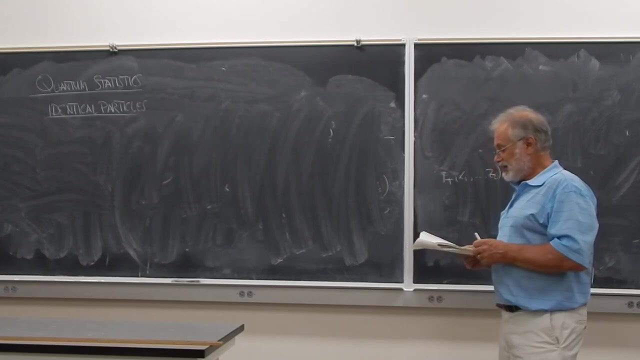 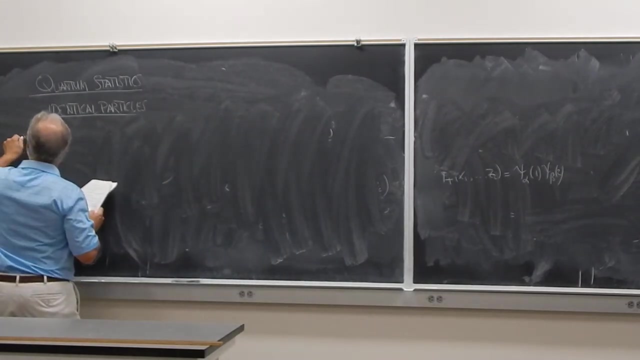 Make it nice and short and sweet. So the question we ask is: do measurable quantities evaluated from psi of t depend on the assignment to particle labels? Let's examine the probability density function. That would be psi sub t star psi sub t. 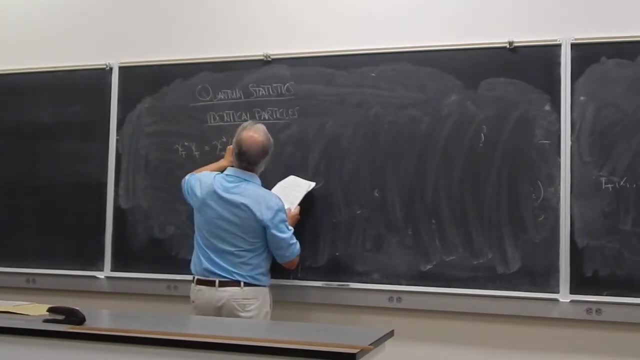 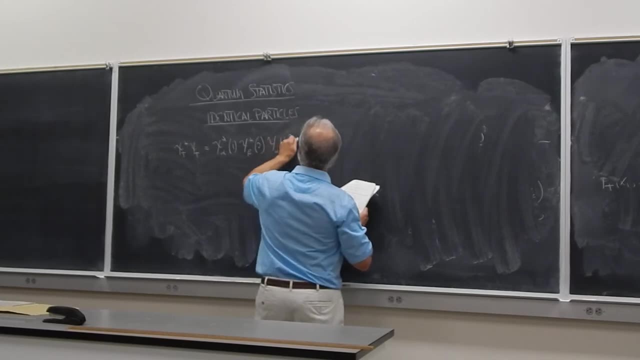 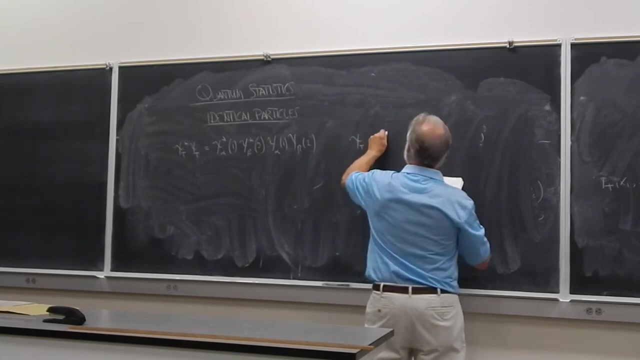 I can write that as psi alpha star of 1., Psi beta star of 2.. Psi alpha of 1.. Psi beta of 2. And that's for psi sub t equal to psi alpha of 1, psi beta of 2.. 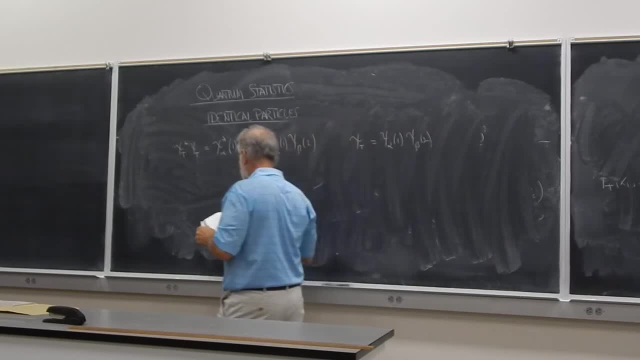 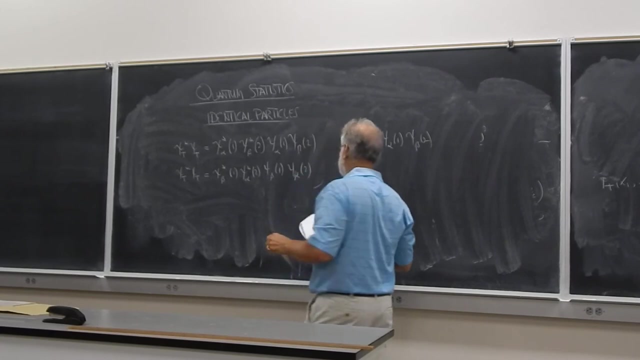 By the same token I can write psi t star, psi t as the product of psi sub t. star of 2.. Psi beta star of 1, psi. alpha star of 2, psi. beta of 1, psi. alpha of 2.. 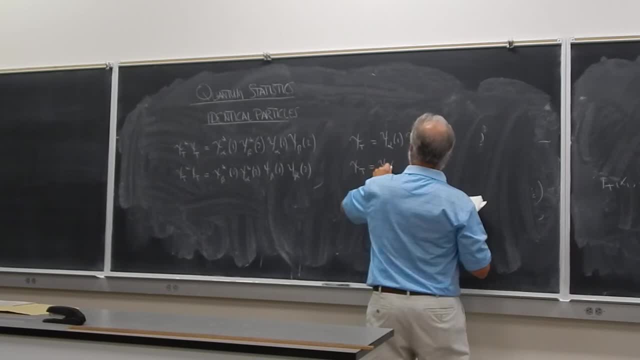 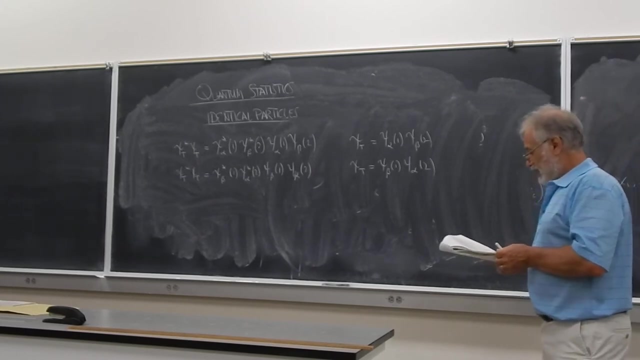 And that would be: psi t is equal to psi beta of 1, psi alpha of 2.. Since the particles are identical, we should be able to exchange the labels without affecting a measurable quantity such as the probability density. Let's see if this is true. 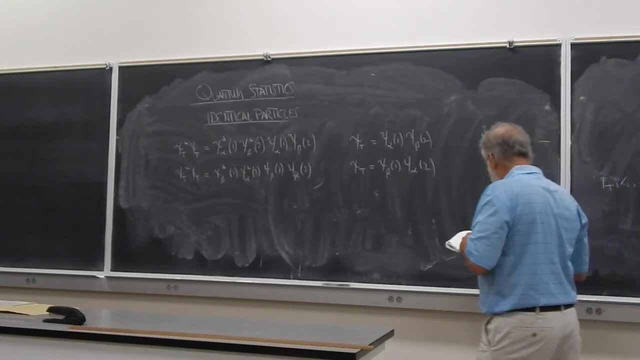 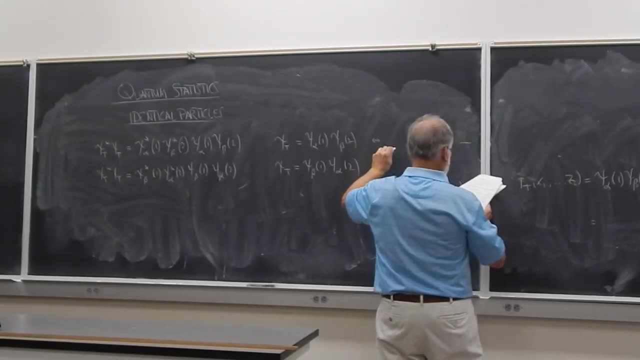 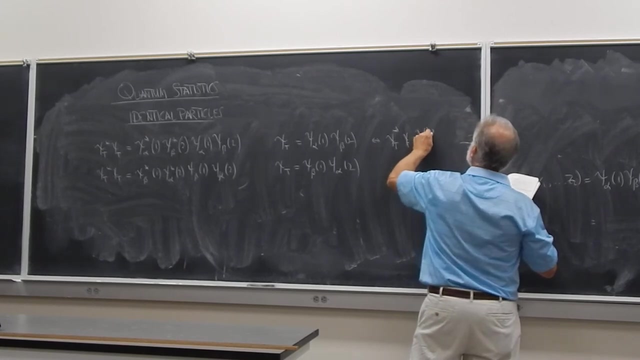 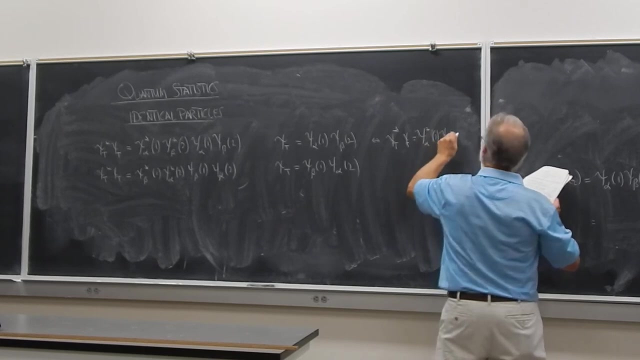 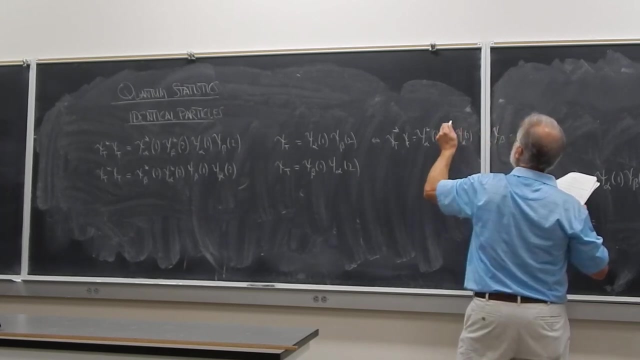 Suppose I exchange labels in the first probability density equation. So if I exchange labels I'm going to get psi t star. psi t is psi alpha star of 2.. Psi beta of 1., Psi alpha of 2.. Psi beta of 1.. 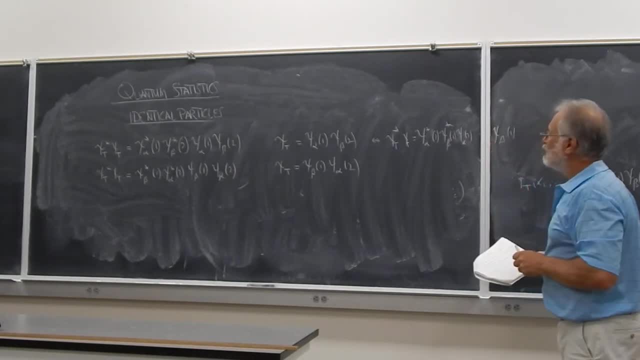 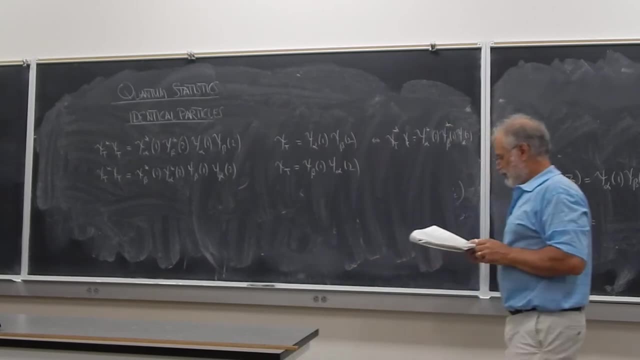 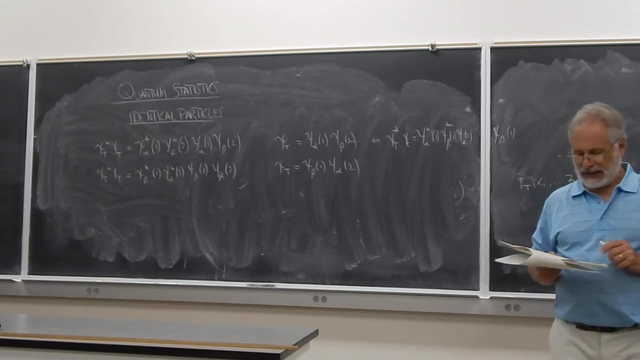 Psi beta of 1.. Notice this new probability density doesn't equal this probability density down. They're not the same. That's a problem. This can only mean that the eigenfunctions we chose, as vanilla as they seem, are unacceptable. 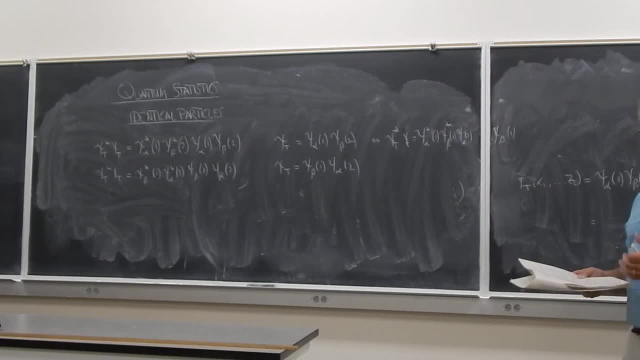 They can't be solutions to the Schrodinger equation because it depends upon how the particles are labeled. Okay, well, we could trial and error a lot of things and spend all day trying to figure out what might be acceptable solutions to the Schrodinger equation. 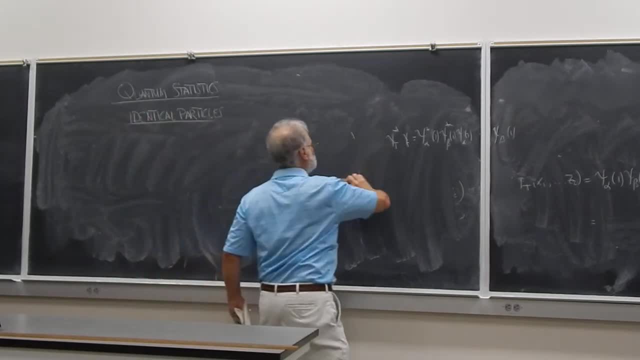 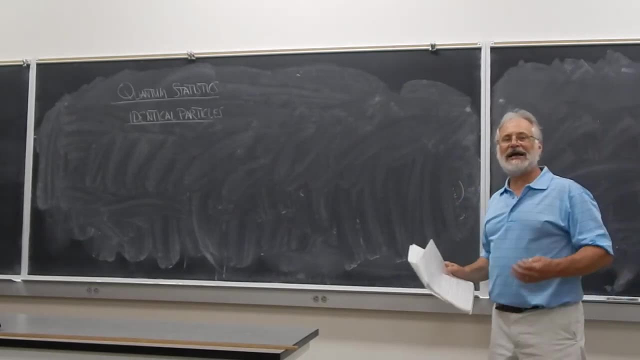 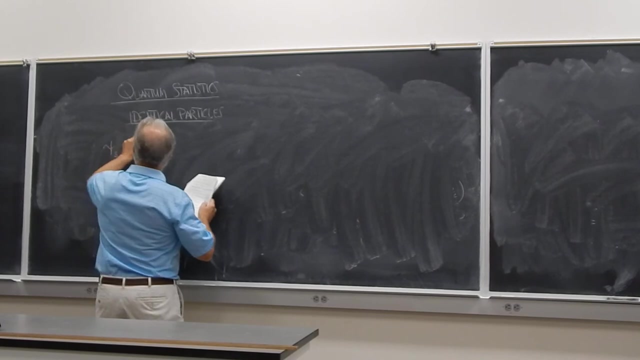 For these electrons. but we won't. We'll cut to the chase and I'm going to show you two eigenfunctions that will work for us. One is called psi sub s, And I'm going to write that as one over the square root of two. 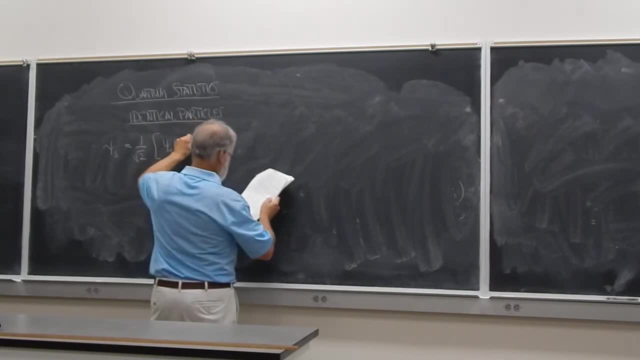 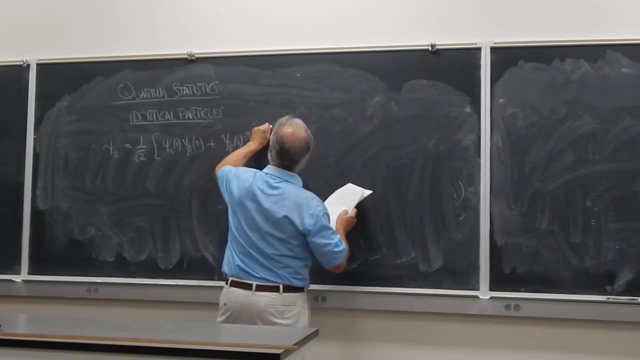 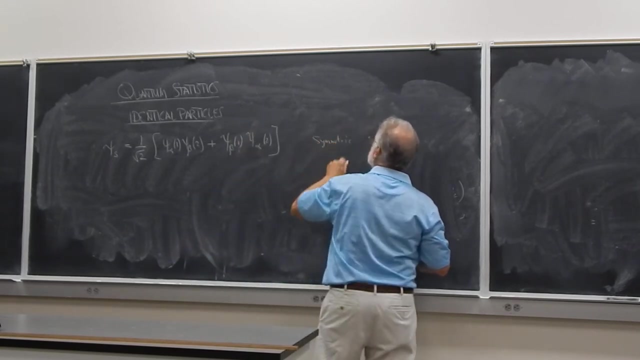 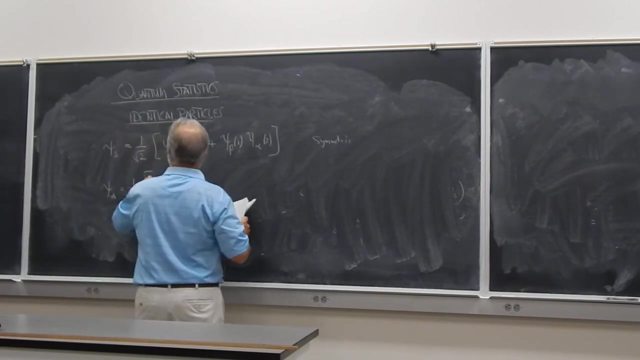 psi alpha of one. psi beta of two, plus psi beta of one. psi alpha of two. This is what we call the symmetric eigenfunction, And I'm going to write psi sub a one over the square root of two. psi alpha of one. 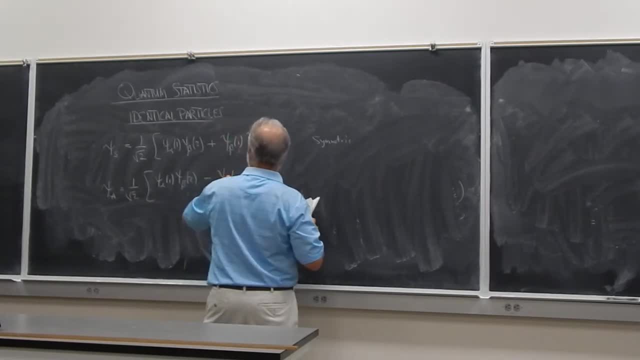 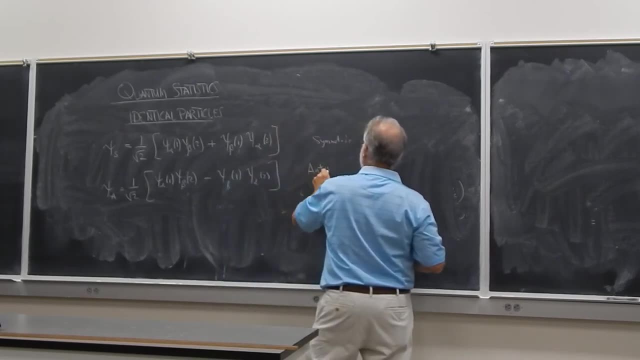 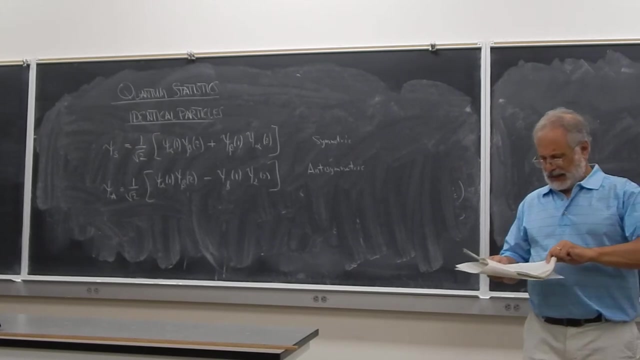 psi beta of two minus psi beta of one psi alpha of two. This is what we call the anti-symmetric Wave function. You might wonder about the square root of two, one over the square root of two, That's to make sure that these eigenfunctions are normalized. 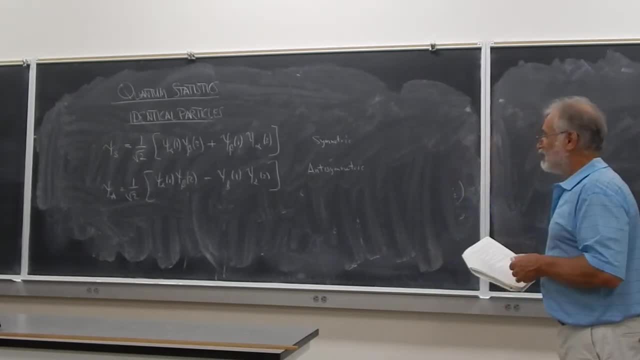 So the total energy of a system containing one particle in state alpha and another in state beta doesn't depend upon which particles in which state. So psi sub t equal to psi alpha. psi one alpha. psi two beta. psi sub t equal to psi one beta. 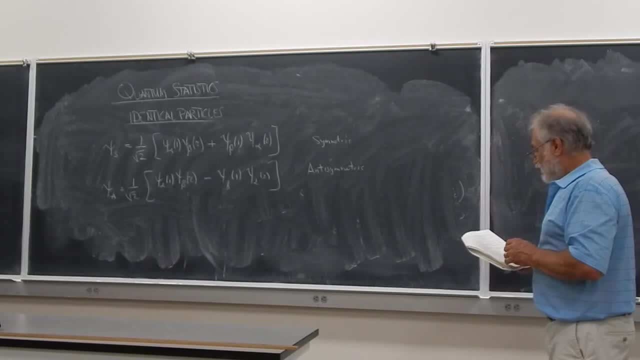 psi. two alpha are solutions which correspond to the same energy, E sub t. Since the Schrodinger equation is linear, linear combinations of my symmetric and anti-symmetric wave functions should also be solutions. In that sense we say that that the solutions to this equation are degenerate. 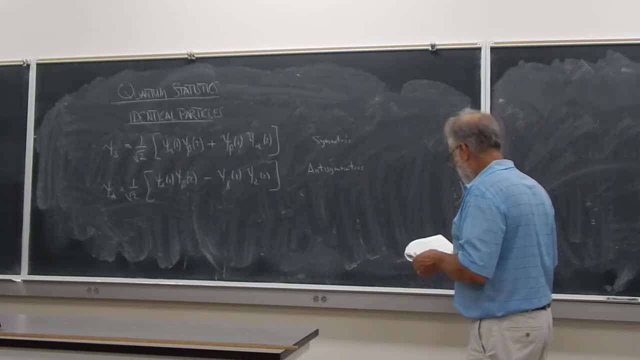 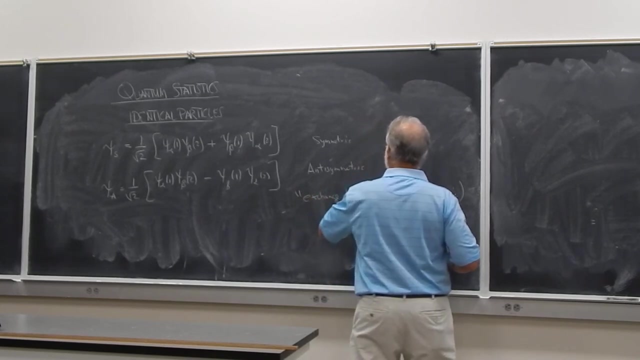 So different eigenfunctions corresponding to the same eigenvalues are what we call degenerate. This is what we call, though this is a particular type of degeneracy. we call this exchange degeneracy because it arises from the fact that it comes from interchanging one particle with the other. 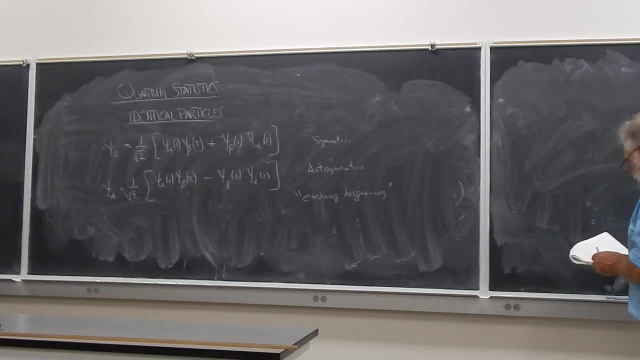 or a particle label. We could also demonstrate that the probability density function would be unchanged under exchange of the eigenfunctions psi s and psi a. For the moment, let's just demonstrate that the eigenfunctions themselves aren't changed. So psi s. 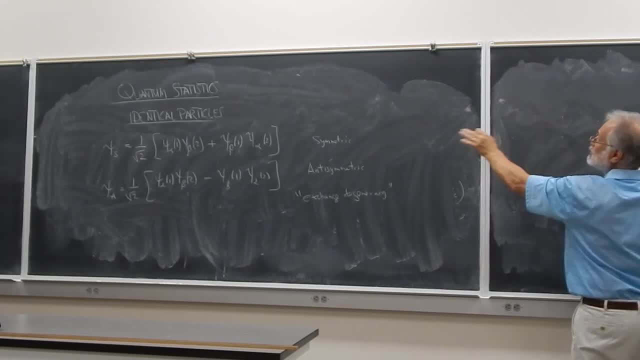 one over the square root of two. now, let's just, we'll use the psi s we have, let's just exchange labels one and two, And what do we get? We get one over the square root of two psi alpha of two. 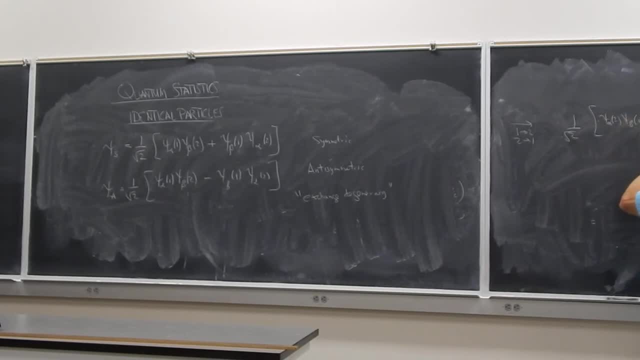 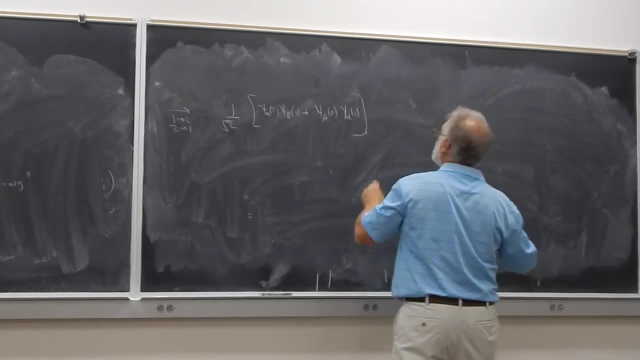 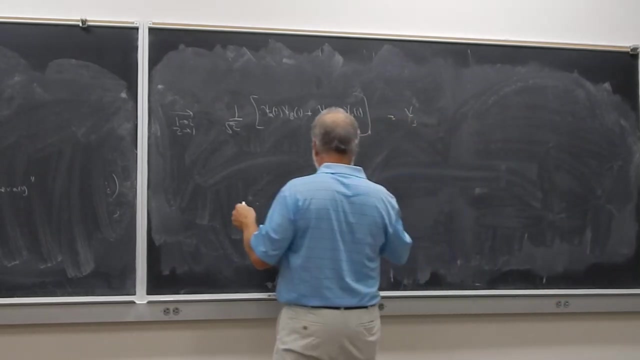 psi beta of one plus psi beta of two, psi alpha of one, which is psi s. So exchanging the labels doesn't do anything to the function. On the other hand, if I do that with the anti-symmetric function, 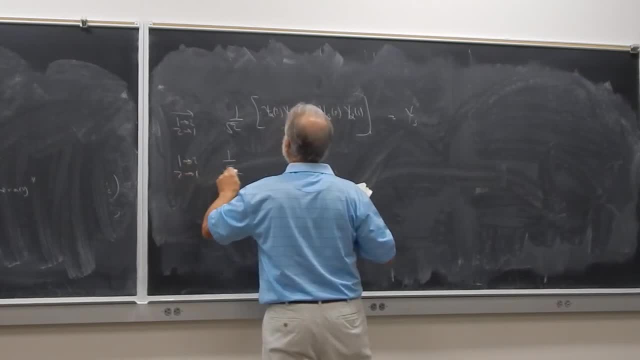 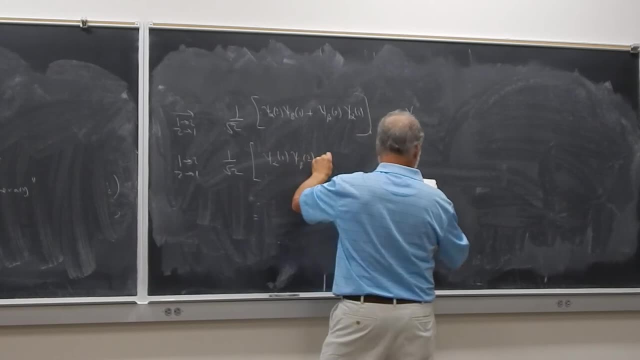 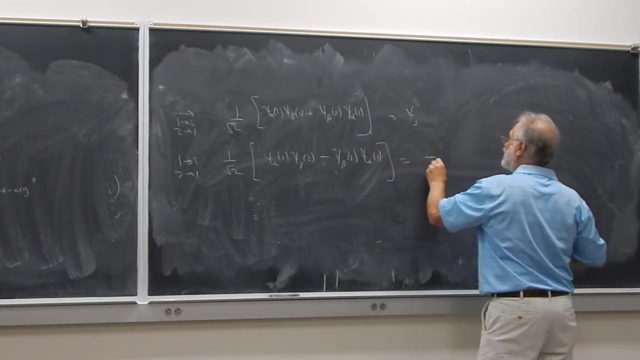 I get one going to two and two going to one. I get one over the square root of two psi alpha of one psi beta of two, minus psi beta of two psi alpha of one. so it's equal to minus the anti-symmetric wave function. 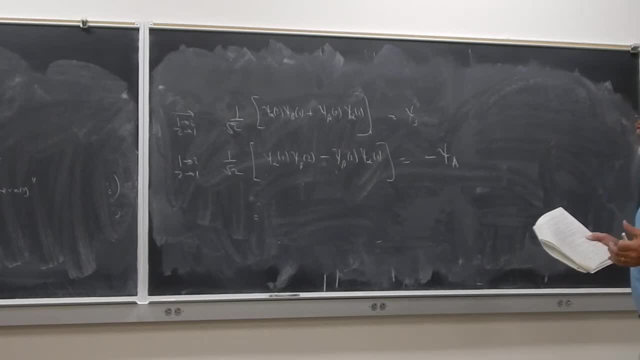 Now, in terms of getting probability density, this is not a problem, because I square them right. I do. psi star psi s star psi is going to be the same as psi a star psi, a. So so far what we can say is: 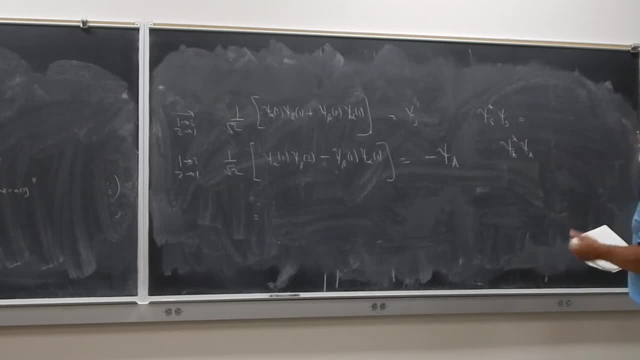 both probability density functions are going to be unchanged by changing the labels, because in this case, if I square this, I'm going to get a positive number anyway. Great, That leads us to the Pauli exclusion principle. According to experimental data, 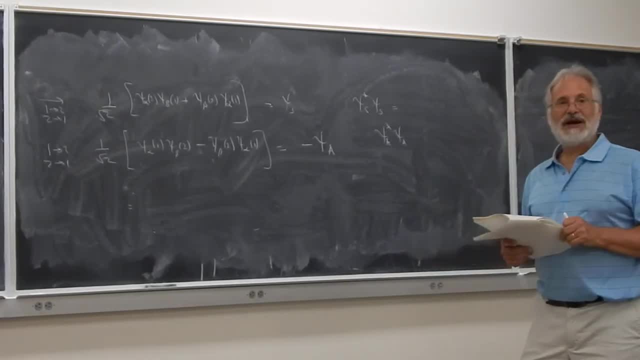 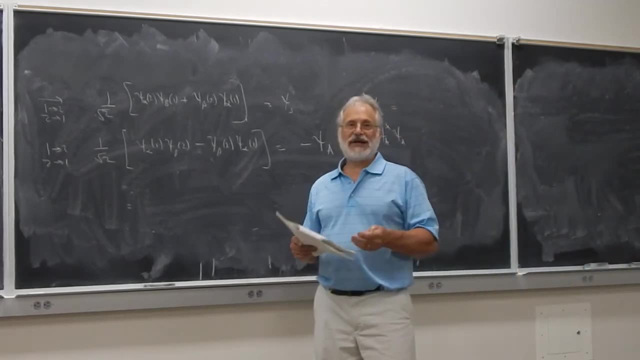 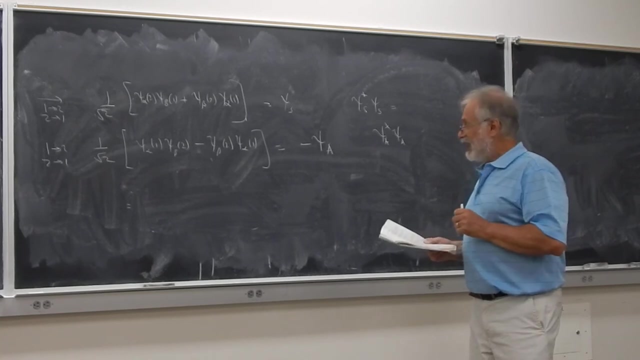 Pauli established that in a multi-electron atom, no two electrons could occupy the same quantum state. This is what we call the weaker statement of the Pauli exclusion principle. Coincidentally, examine the anti-symmetric eigenfunction that we just derived. 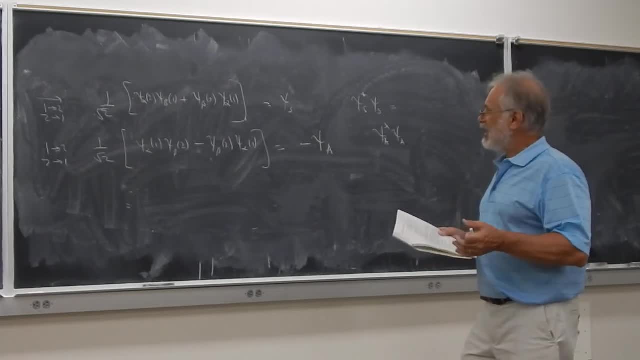 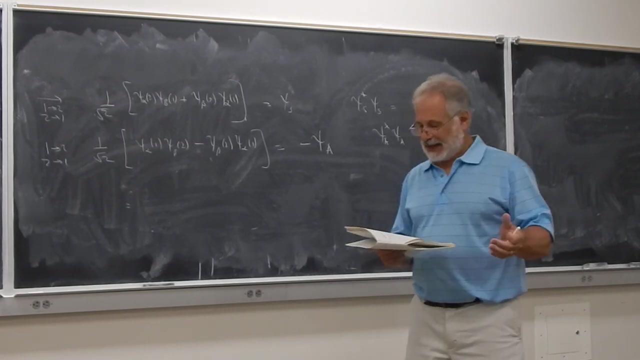 If the particles in that case occupied the same state, the eigenfunction would be zero. So what this is saying is two particles described by an anti-symmetric function can't both be in the same state, They can't have the same spin. 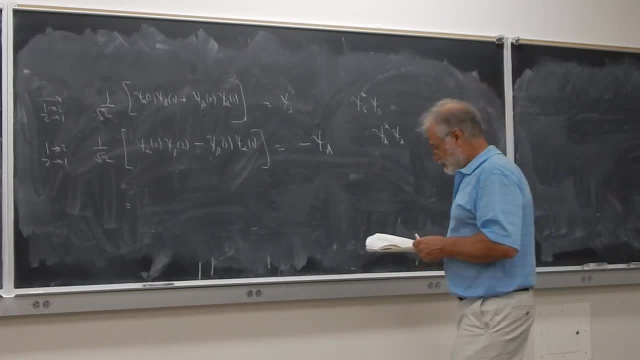 and space quantum numbers. So another way of saying this is that all anti-symmetric eigenfunctions will obey the Pauli exclusion principle. A system that has several electrons has to be described by an anti-symmetric total wave function. That's what we call. 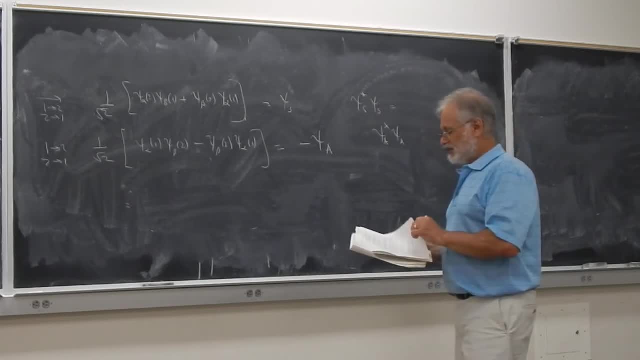 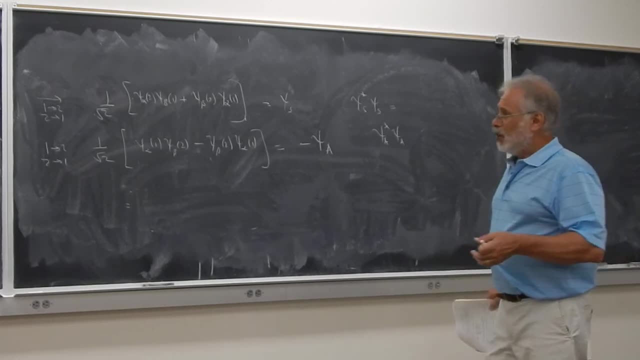 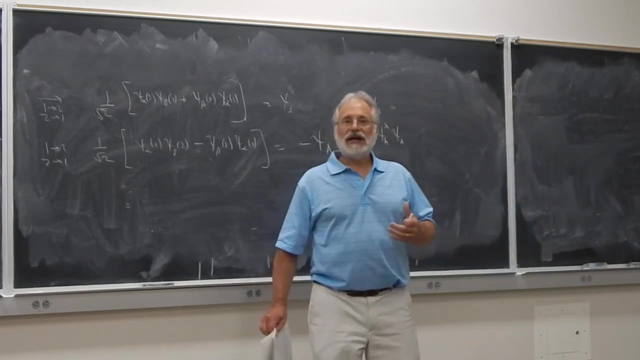 the strong form of the Pauli exclusion principle. Symmetric and anti-symmetric eigenfunctions are going to lead us to two different types of statistics. What we plan to do in the first part of this unit is to actually look at three types of statistics. 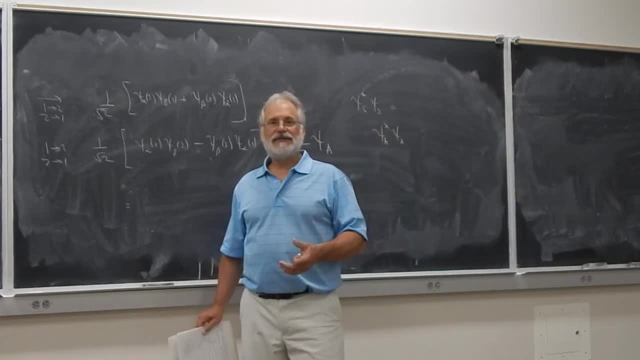 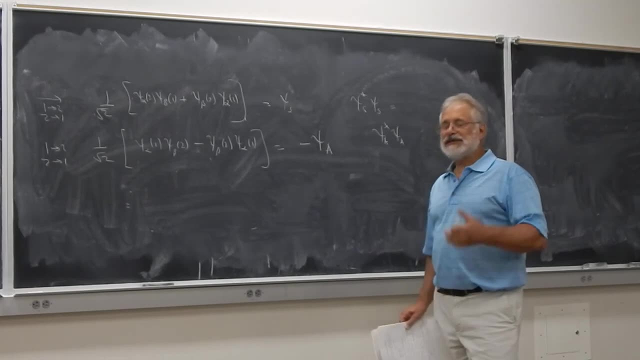 We're going to look at Fermi-Dirac statistics which use anti-symmetric wave functions. We look at Bose-Einstein statistics which reflect symmetric wave functions, And then we're going to, as a comparison, look at Maxwell-Boltzmann statistics. 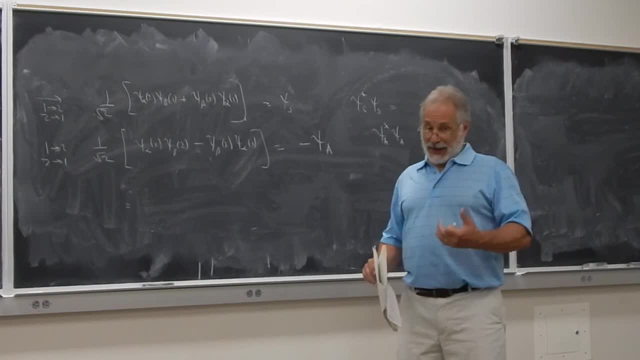 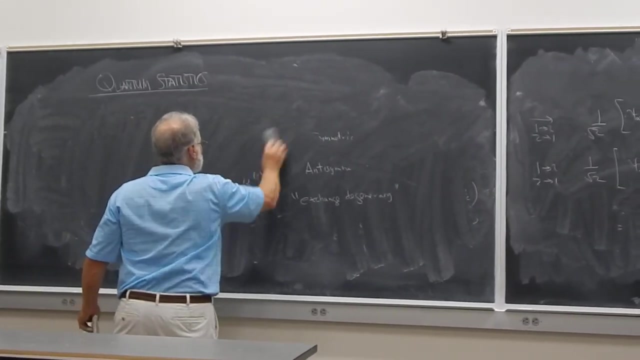 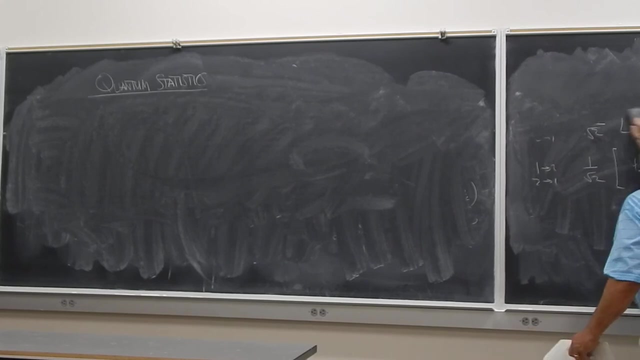 the statistics that we did classically to use as a comparison for both of those systems of statistics, You wouldn't think that a plus or minus sign would make such a difference. But as you'll see as we study quantum statistics, that plus or minus sign 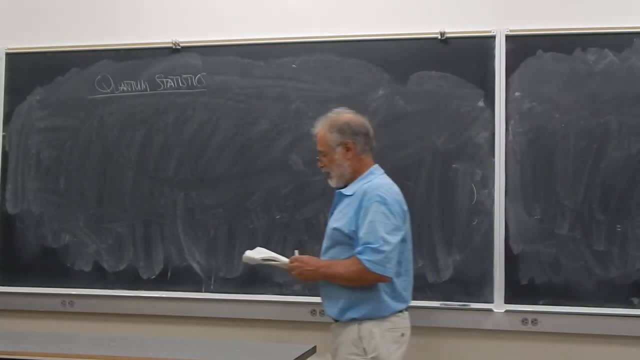 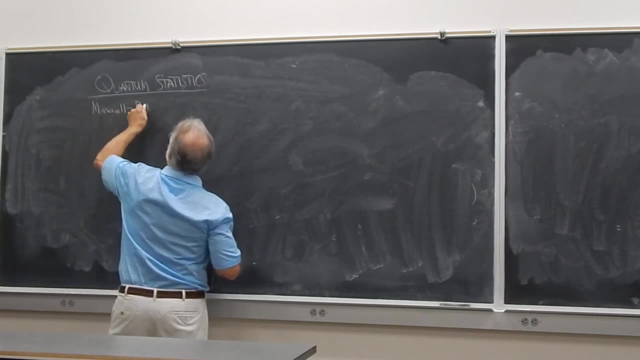 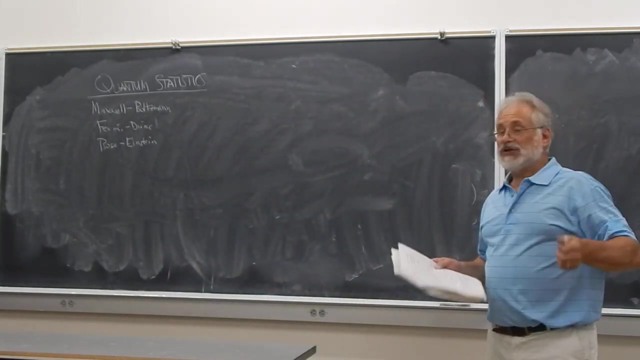 makes a world of difference. So, as I say, as a comparison, we use Maxwell-Boltzmann statistics, we will use Fermi-Dirac statistics and we will use Bose-Einstein statistics. We're dealing solely with identical particles here. 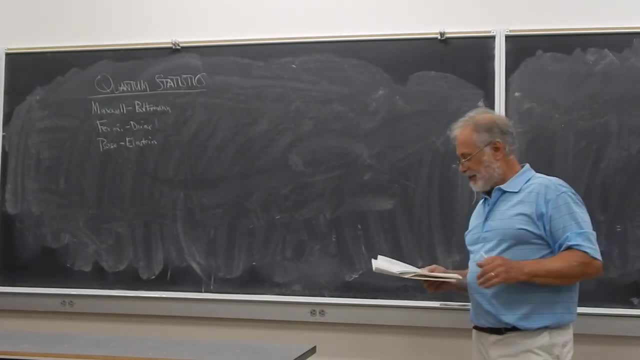 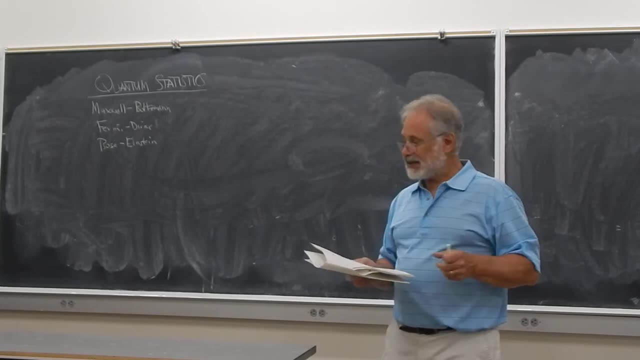 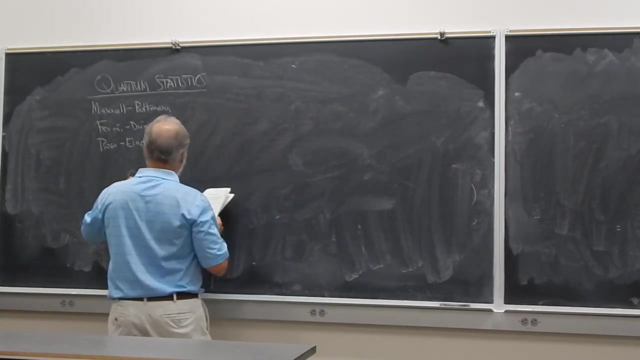 particles where you can't tell one from the other. The system that we're going to be interested in the old. let's take a gas of n identical particles contained in a container of volume V and we'll use Q sub i to designate the particle position. 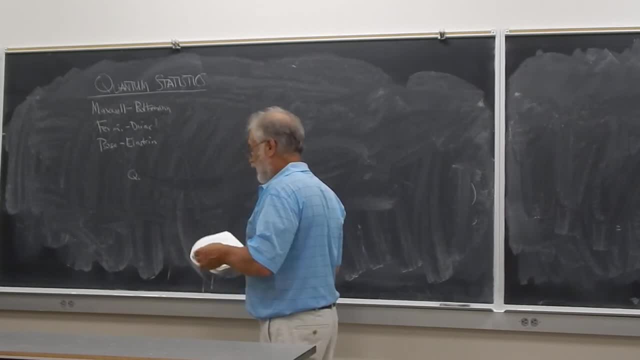 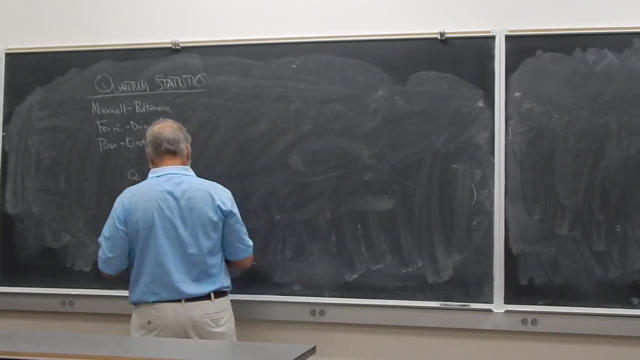 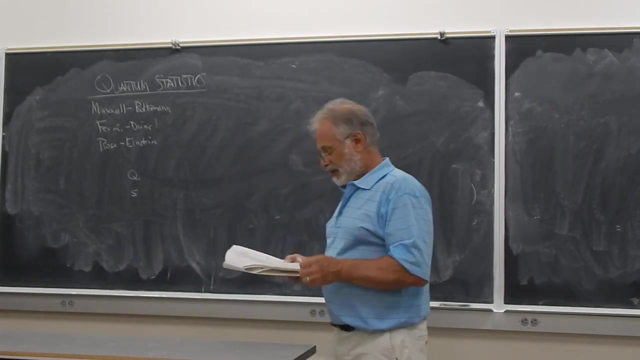 of the i-th particle. P sub i would represent the particle momentum of the i-th particle And we'll use s to label the state of that particle. So what we're going to do, put them all together and we're going to be looking for. 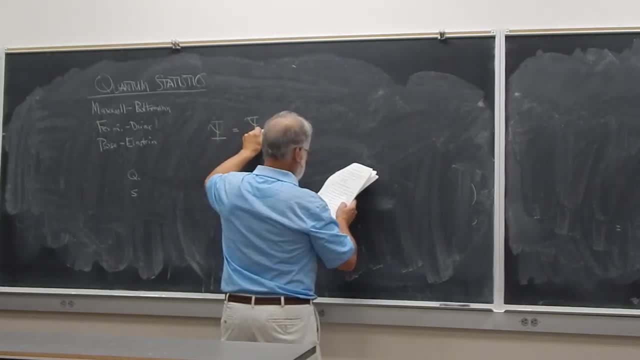 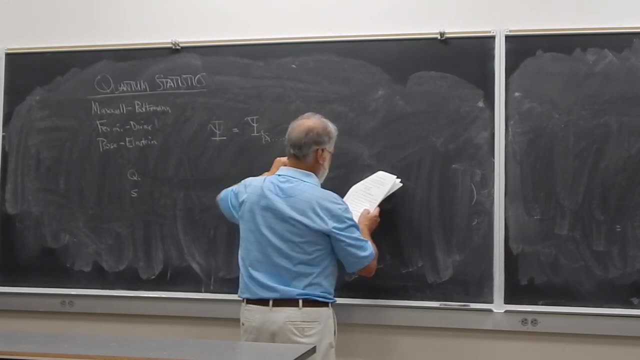 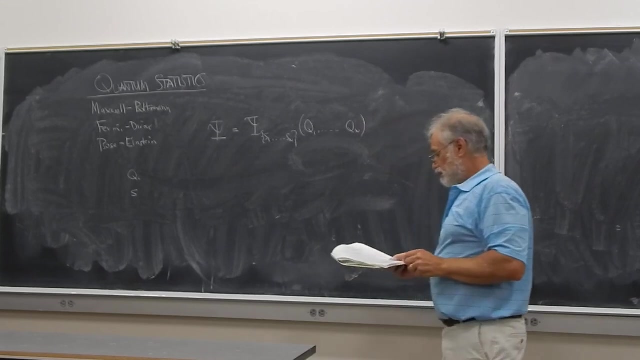 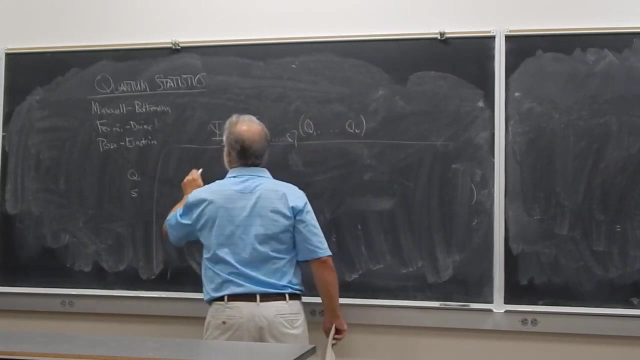 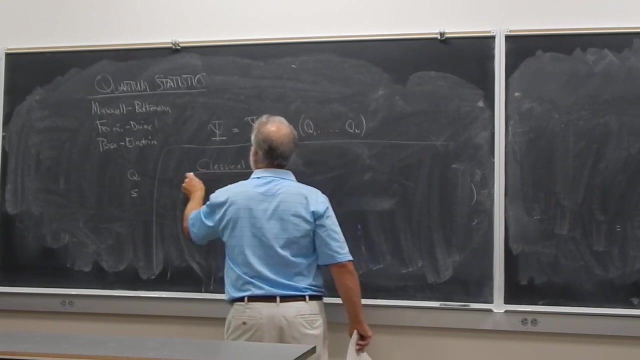 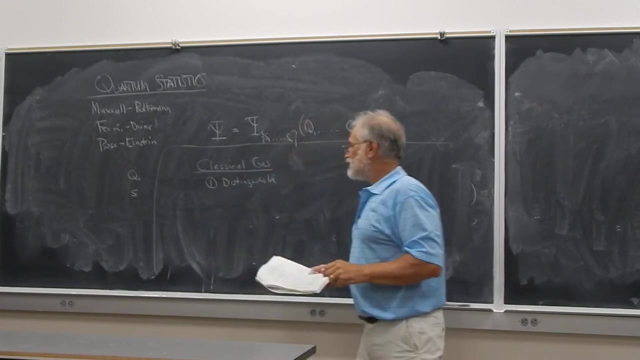 a wave function, that is, a function of a collection of states, one through n, and of positions. Okay, Let's just again- this is for comparison's sake- start with the classical gas. First thing we know, Boltzmann statistics, classical gas. particles are distinguishable. Two: there's no limit on the number of particles in a state. You can have as many particles as you like in the same state. So we don't obey the Pauli exclusion principle with this kind of statistics. 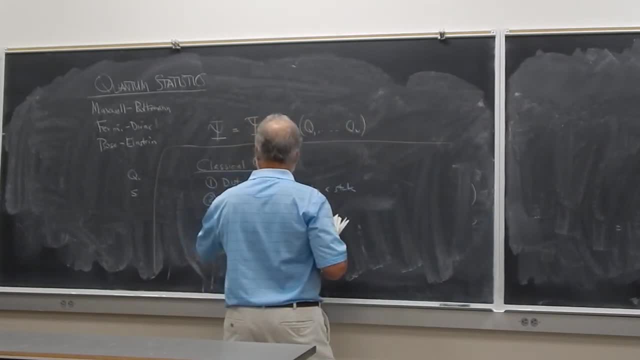 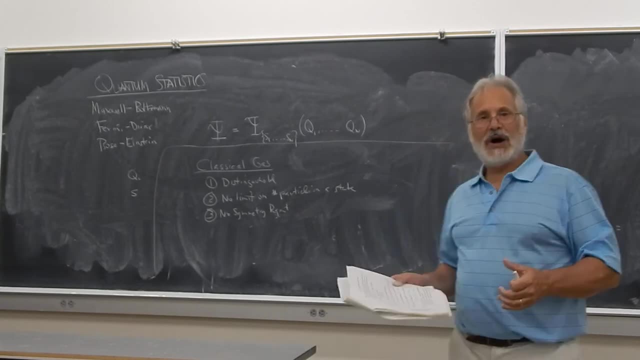 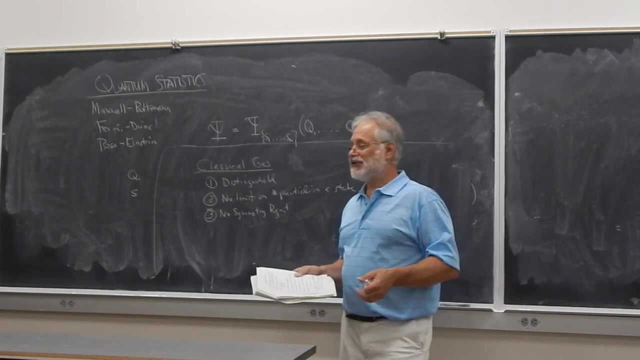 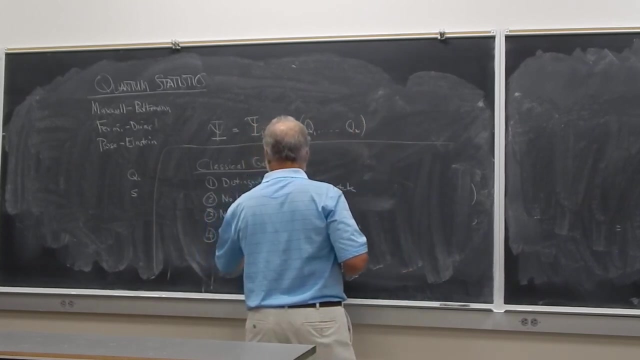 Three, there's no symmetry requirement at all. Remember, we in quantum statistics, when I have identical particles, I either have anti-symmetric or symmetric wave functions. There's no symmetry involved in classical statistics And, of course, obviously, when it comes to quantum mechanics. 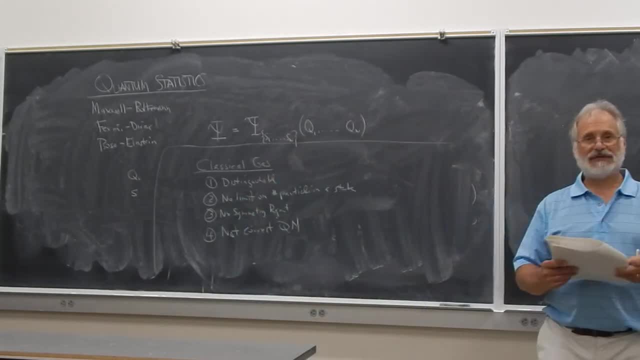 it's totally not correct. Again, we're just using it for comparison. If I want to use quantum mechanics, I have to impose symmetry requirements under the interchange of any two identical particles. You don't get a new state when you interchange two of these particles. 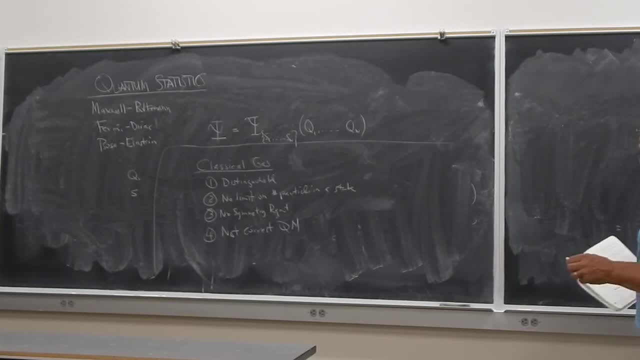 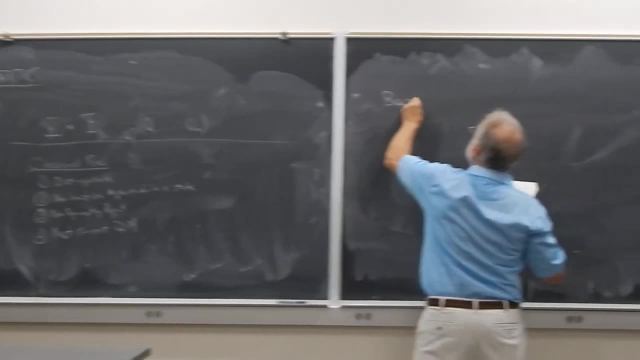 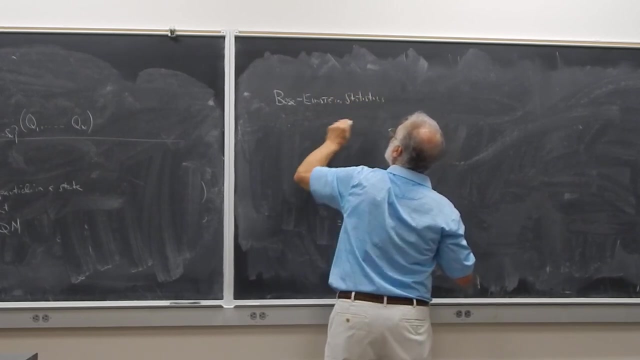 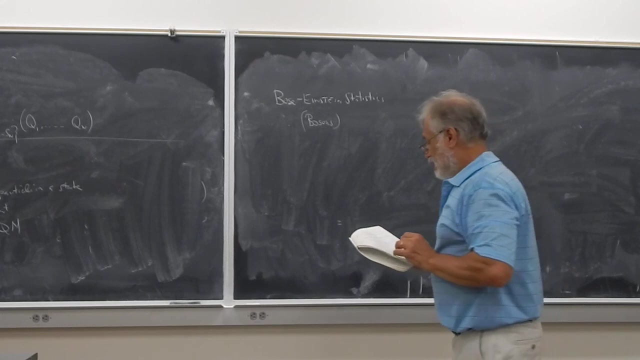 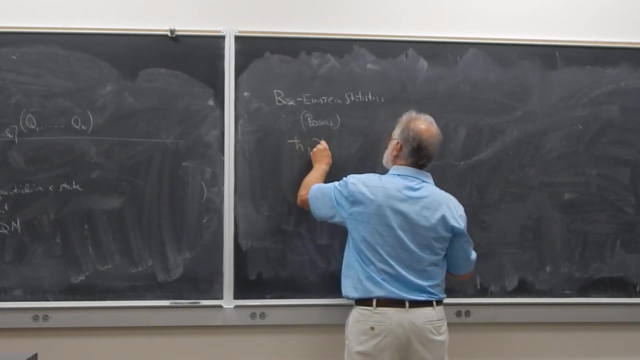 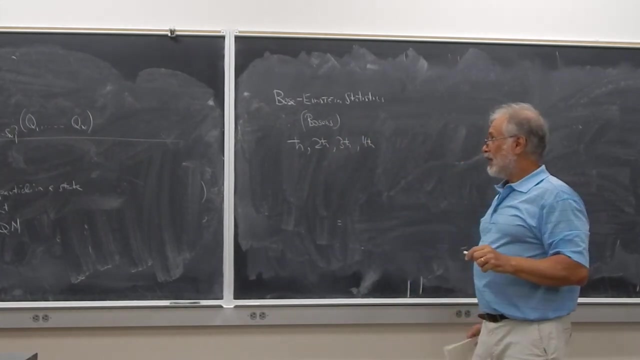 And you wouldn't expect it. So the second case would be what we would call Bose-Einstein statistics. We call these particles bosons. What are the characteristics? Each particle has a total spin, angular momentum of integral multiples of h bar. Examples of bosons. 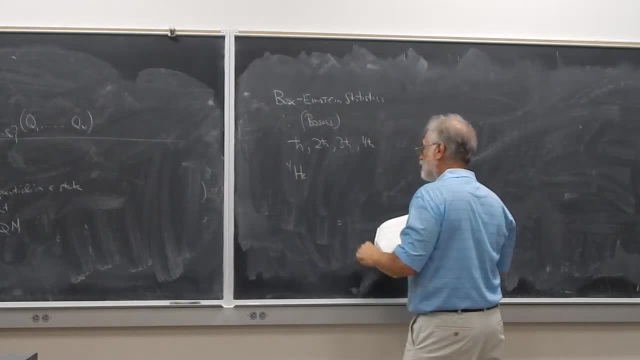 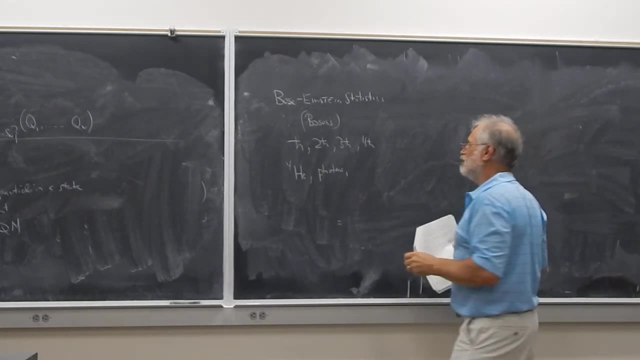 The helium-4 atom Photons, For those of you who like to study the standard model, the W plus minus and the Z boson, the neutral Z boson in the weak force, Gluons, All these gravitons. 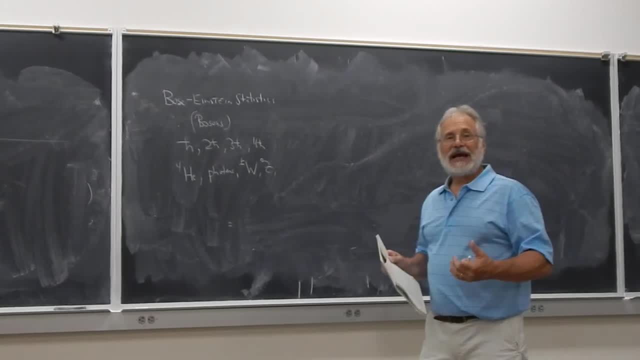 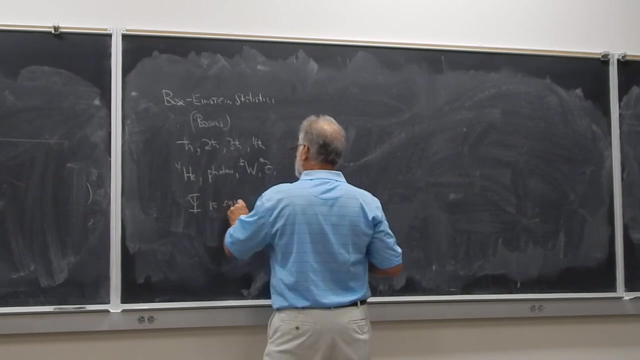 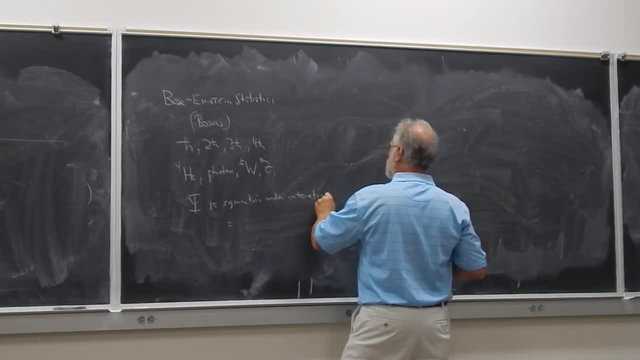 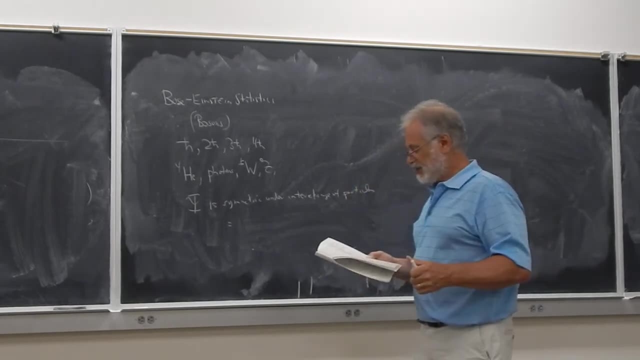 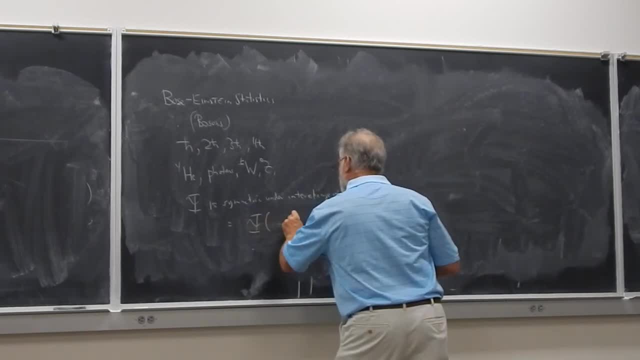 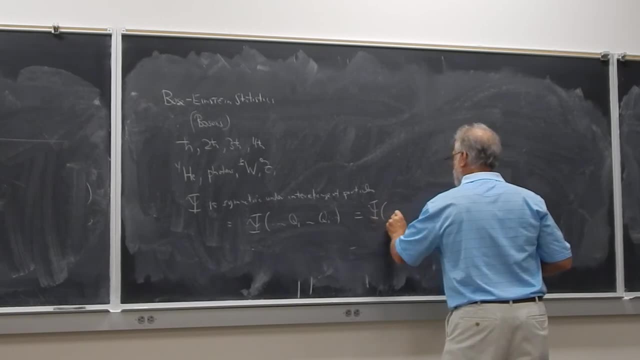 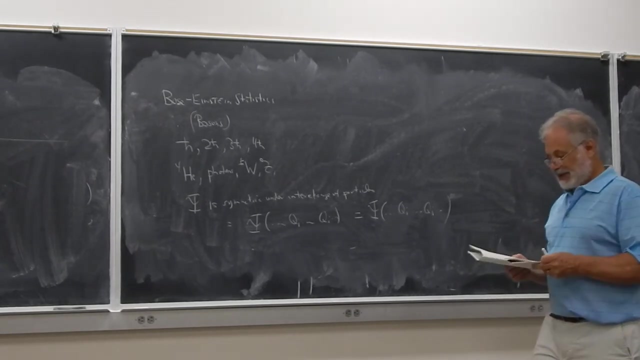 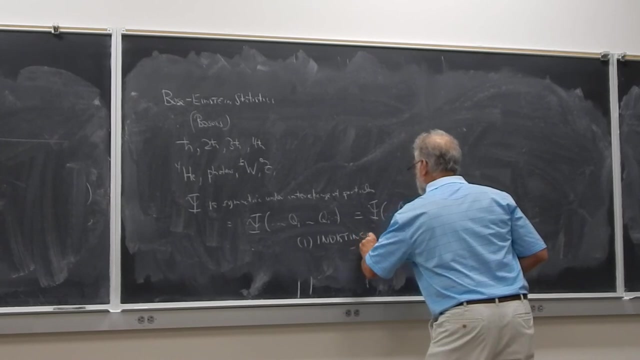 if I want to put it symbolically, Psi of whatever Q sub j, Psi is symbolَ. If I want to say Khan, or cutting set, Well, we said, interchange of these two particles doesn't lead to a new state of the gas, That must mean one. I can't tell one from the other. Particles are indistinguishable. As I said, that's characteristic of quantum statistics. No limit on how many occupy a state, No limit at all. We call these guys bosons. They obey Bose-Einstein statistics. Last type: Fermi-Dirac statistics. 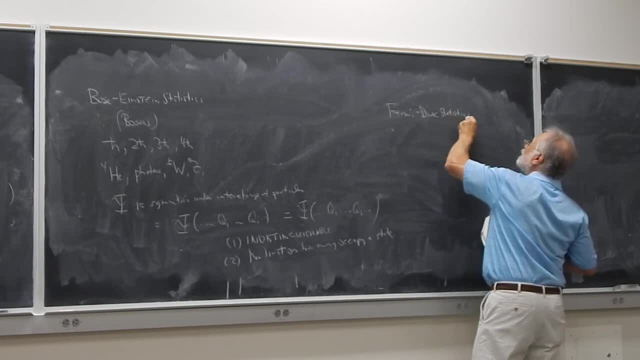 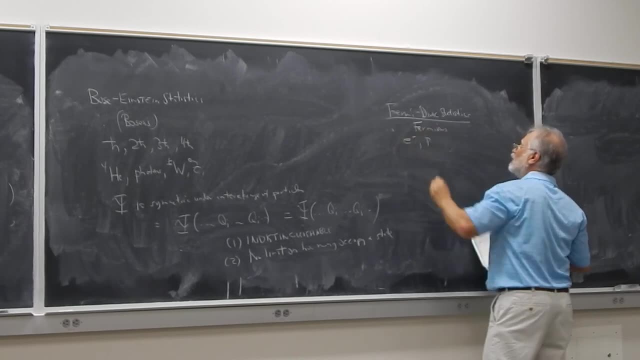 Okay, Okay, We call these guys fermions. Good examples: electrons, protons, all the hadrons that you can think of- are all fermions. They have half-integral spins. so h-bar over 2, 3h-bar over 2 are the allowed spins for. 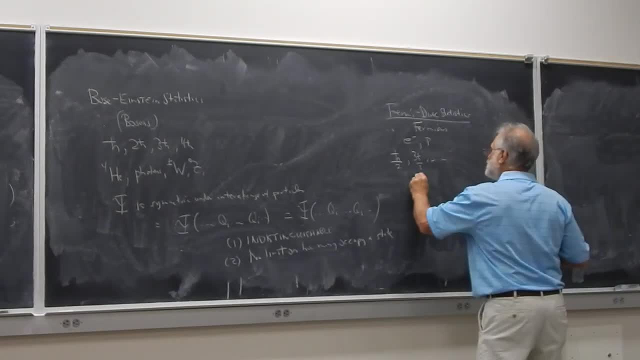 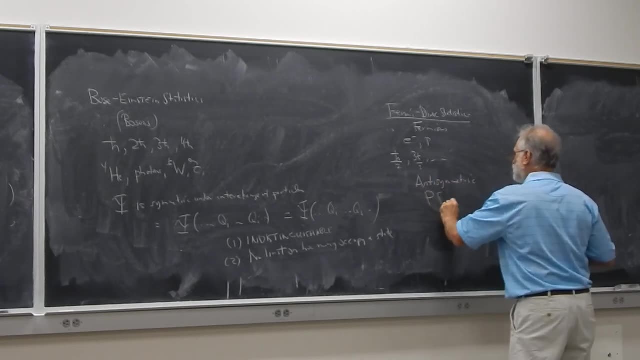 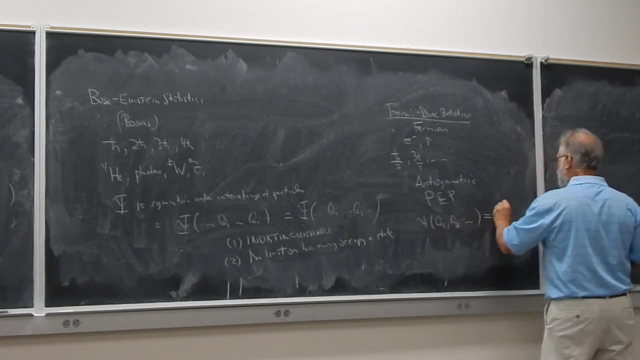 fermions. The symmetry requirement is that they must be anti-symmetric. They must be described by anti-symmetric wave functions. They obey the Pauli exclusion principle and so they're going to be. if I interchange two particles, psi of q1, q2, etc. is equal to minus psi of q2, q1, so anti-symmetric and 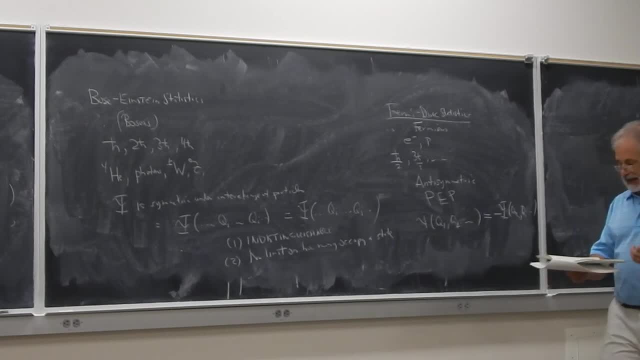 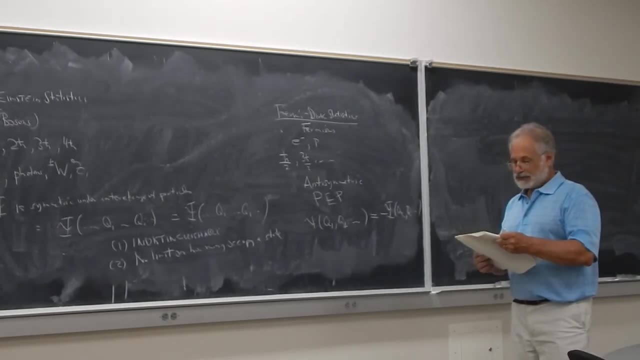 I'm only allowed to put one particle in one particle state, So I'm obeying the Pauli exclusion principle that says only one particle can occupy one state. These guys are also indistinguishable. We're going to pick up with this and the characteristics of these systems in the next lecture. Thank you.